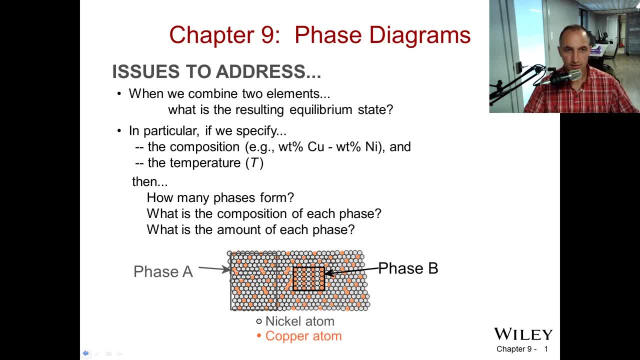 Good afternoon everyone. This is Eric Payton Introduction to Materials Engineering, Chapter 9, Phase Diagrams- Issues to address today. when we combine two elements, what is the resulting equilibrium state? In particular, if we specify the composition- weight percent copper and weight percent nickel- and the temperature? 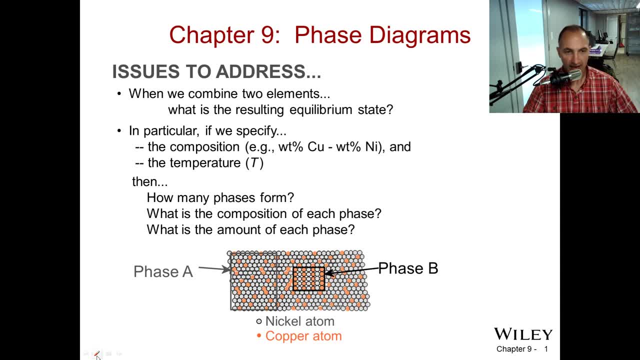 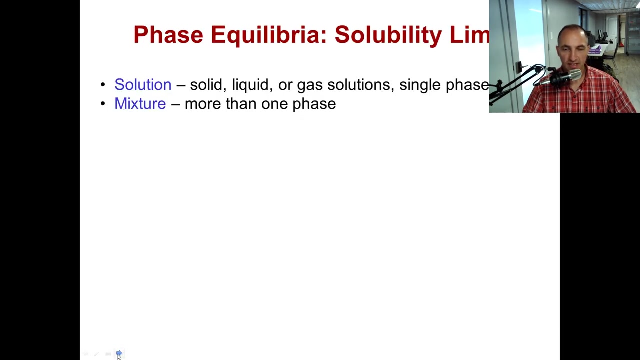 then answer the questions: how many phases form, What is the composition of each phase And what is the amount of each phase, the weight percent of each phase? Okay, so phase equilibria and solid solubility. So a solution is just a solid liquid or gas solution and it's a single phase. 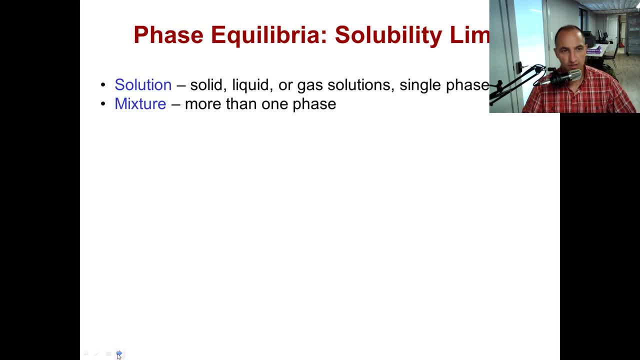 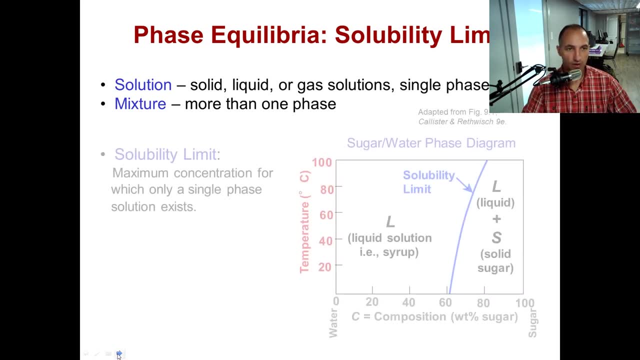 A mixture, however, is more than one phase And the solubility limit is just the maximum concentration for which only a single phase solution exists. So in this example, let's ask the question: what is the solubility limit for sugar in water at 20 degrees C? 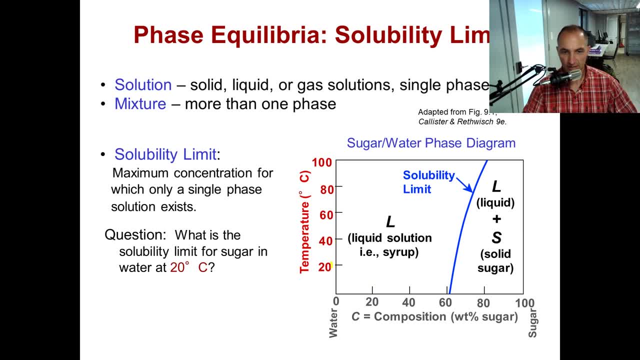 Okay, So we're looking at this temperature right here And what is the solubility for sugar at 20 degrees. So we just move across here to the boundary and we go down to the composition. So the composition is 65.. 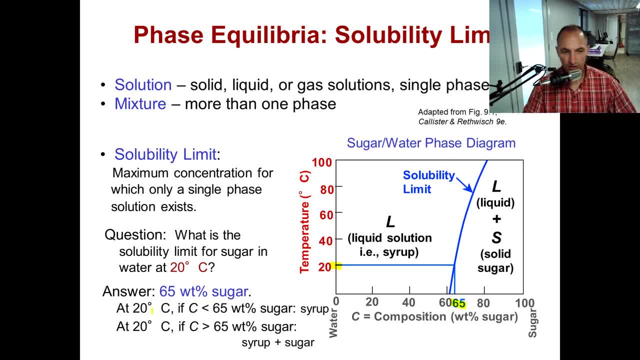 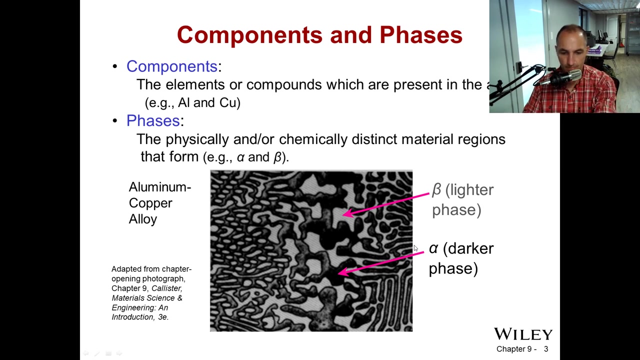 So the answer is 65 weight percent of sugar And at 20 degrees C. if the composition falls below 65 weight percent, you're going to go to a syrup. If you go above 65, you're going to have a syrup. plus, you're going to have some solid sugar. 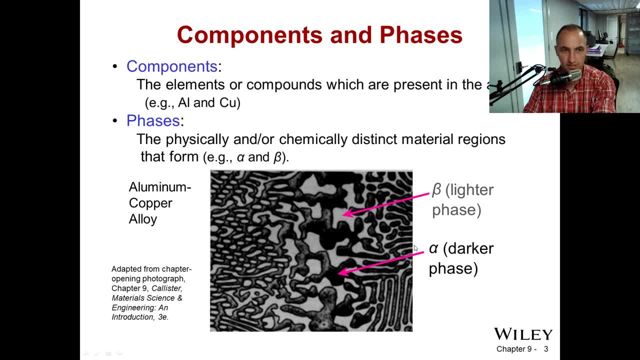 So components and phases, This is just terminology. now, Components are the elements or the compounds which are present in the alloy. So aluminum and copper are components in this system. Now the phases that are present, these are the physical and or chemically distinct material regions that form. 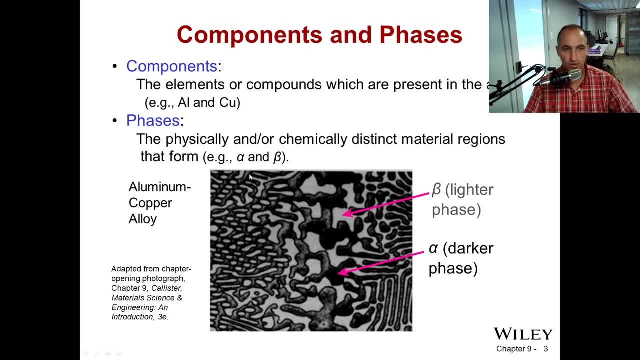 In this example, this aluminum and copper alloy, the phases are alpha and beta, So the term phase is not just confined to phases of matter like gases, liquids, solids and phases. Those are the four main phases of matter, But this definition is a bit broader than that. 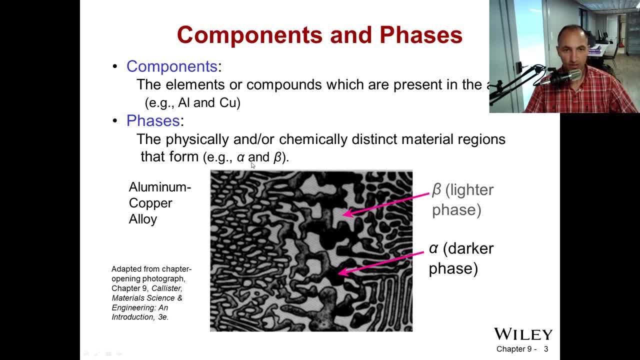 The phases may be identical in chemistry But we might have a different physical structure, like a different crystal structure. for example, Alpha phase is copper rich and you have a beta phase which is aluminum rich in this case. So the beta is light and the alpha is this dark phase. 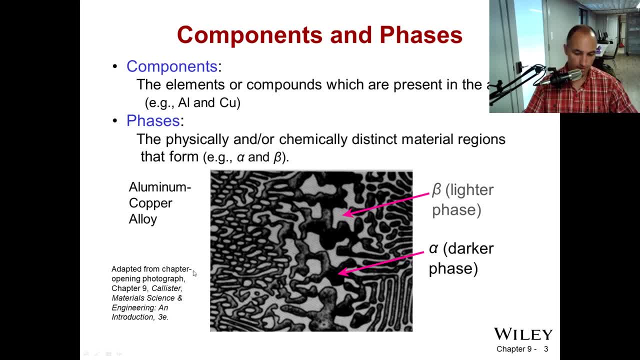 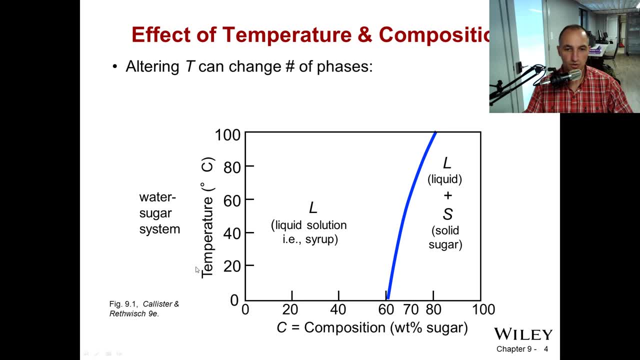 All right, So the effects of temperature and composition. So we're back to the simple sugar water phase diagram. Now let's try altering the temperature, And this can change the number of phases present. Let's take a path from point A to point B. 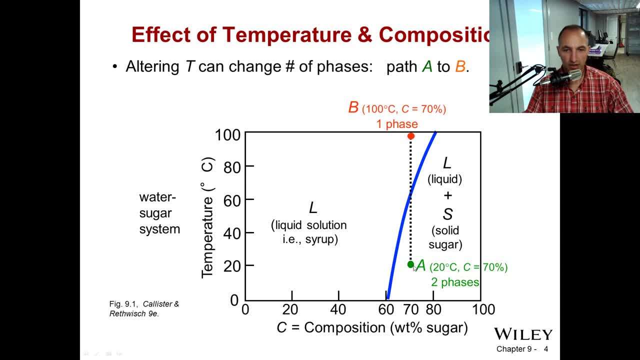 So we start out at 20 degrees C and a composition of 70% sugar in the water. We leave that composition constant, but then we raise the temperature of that two phase And we can end up with 100% syrup or liquid solution here at B. 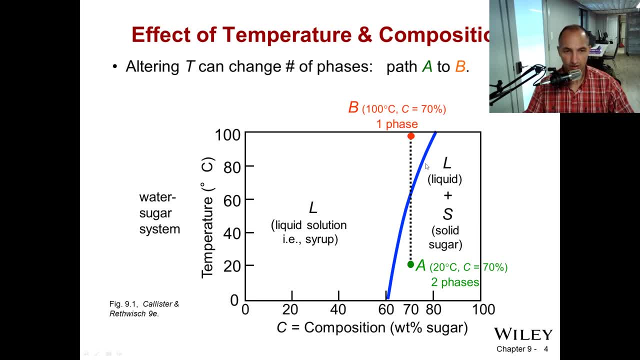 So at 100 degrees C at the same composition, we have all syrup again. So now let's take that path from B and go back to D. Now we can go back into the two phase region of liquid plus solid. Oops, And liquid plus solid. we are at 90%. 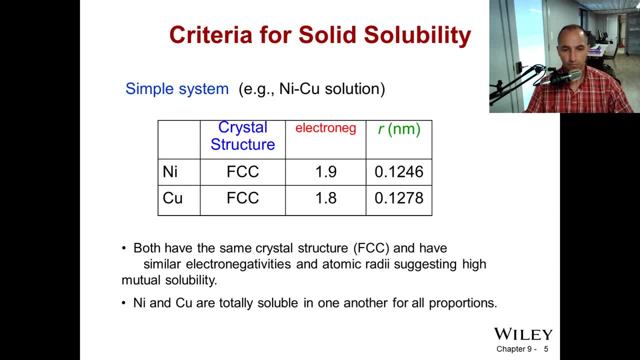 And we're back into two phases. So the criteria for solid solubility: simple system here with nickel and copper, As we discussed in previous chapter with the Hume-Rothery conditions, if we have similar or I should say the same crystal structures here. 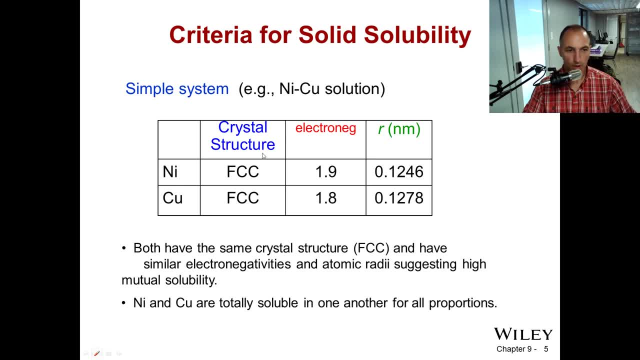 Oops, Same crystal structures And they're both FCC. And very similar electronegativities- 1.9 and 1.8.. And very similar atomic radiuses- Both these. these are all close enough to where we can get high mutual solubility. 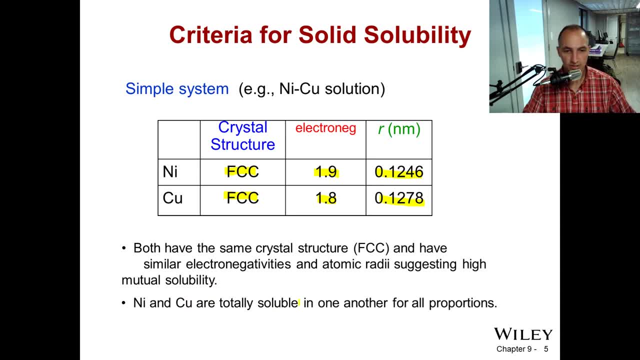 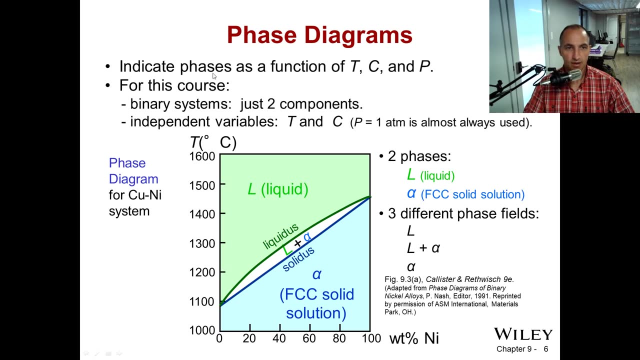 And so, in fact, nickel and copper are totally soluble in one another, And this is for all proportions of nickel and copper together. So phase diagrams indicate the phases as a function of temperature, composition and pressure. P is pressure. However, for this course we're going to look at binary systems. 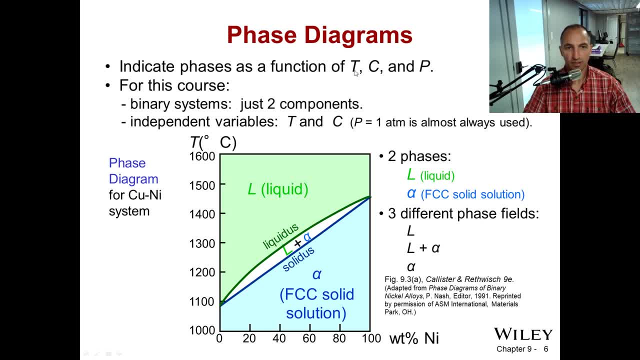 So we're only looking at just two of these three components. So we're only looking at temperature and composition, And we are disregarding the pressure. We're assuming that we're at one atmosphere for all of this. So this is called a binary system. 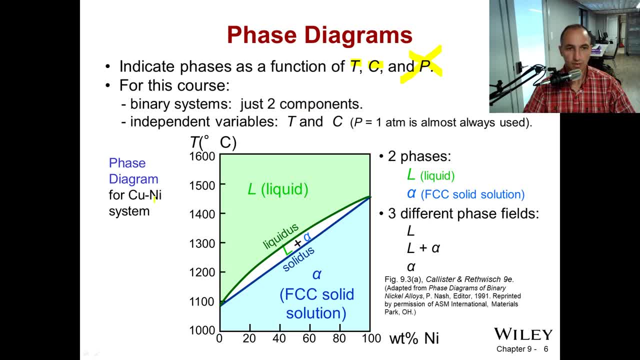 Binary system, two components, And this is what the phase diagram looks like for copper and nickel, And so on the x-axis here, on the far right we have 100% pure nickel And on the left we have 100% pure copper. 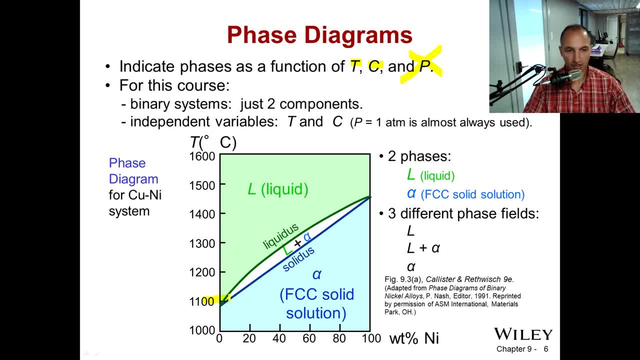 So this is the temperature of, this is the melting temperature of pure copper And this is the melting temperature of pure nickel. Just by going down through here, it goes from liquid to solid at that temperature. So there's two phases In this. there's a liquid. 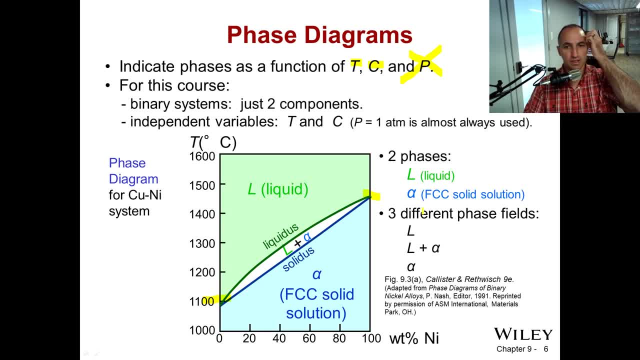 And then there's an alpha And that's it. But there are three phase fields. We can have a liquid, We can have a liquid plus alpha And then we can have just alpha. So this white region in here is kind of like a slushy zone here. 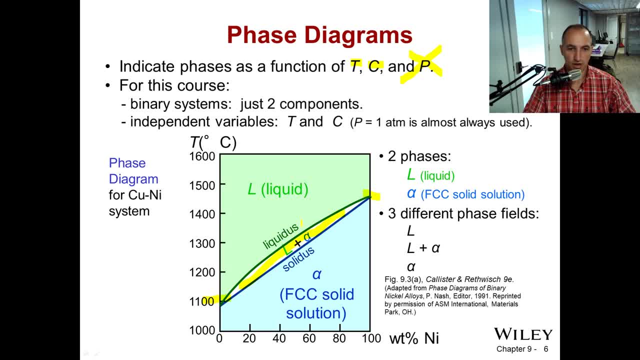 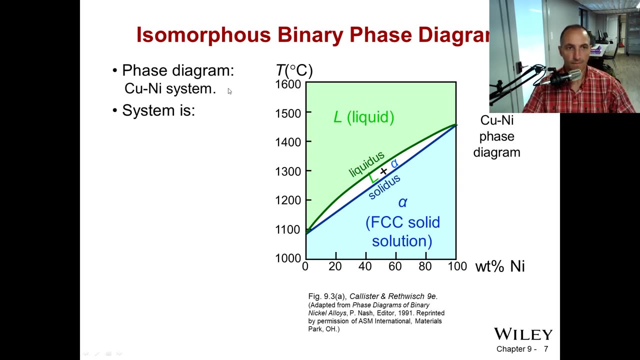 where it's partially liquid and it's partially solid And then, as you cool, then that slush goes to 100% solid. Another term here to introduce is isomorphous. So isomorphous just means that we have a single phase. 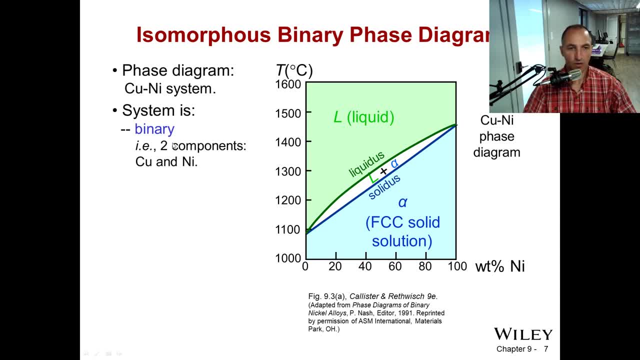 And the system is binary. We have two components, Copper and nickel, And so isomorphous again means that we have complete solubility of one component in the other. Single alpha phase exists all the way from zero to 100% nickel. 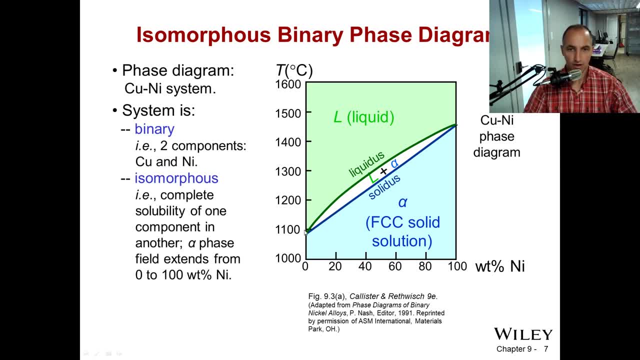 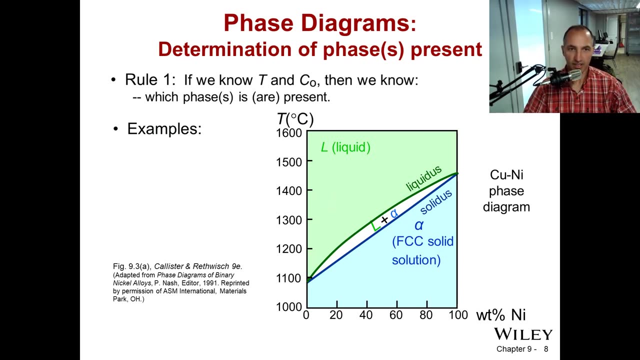 This alpha phase exists all the way across here. We don't have any other solid phase that we're introducing to the system, So this is what we call isomorphous. Now on to the phase diagrams. We're going to determine the phases present. 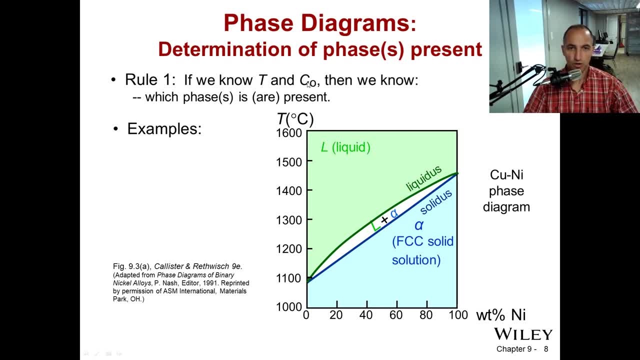 Rule number one is: if we know the temperature and we know the C zero, which is the overall- O stands for overall composition- then we know which phases are present. Let's look at this as an example, At point A, which is at 1,100,. 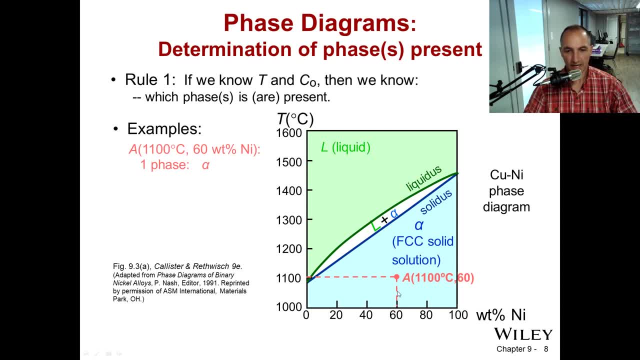 and at 60% weight percent nickel. that means it's 40% of copper, by the way, So it's got 60 of nickel. At this point A we have a single phase, which is alpha. Another random point here: 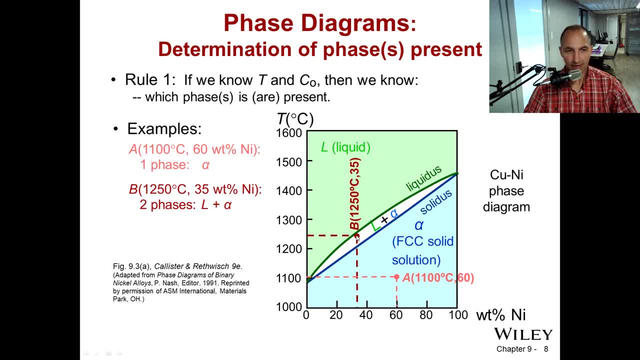 I'm just pulling up is at point B, which is at a higher temperature, at 1,250 degrees C, and it has a weight percent nickel of 35% In this region. here we have two phases. We have liquid and alpha. 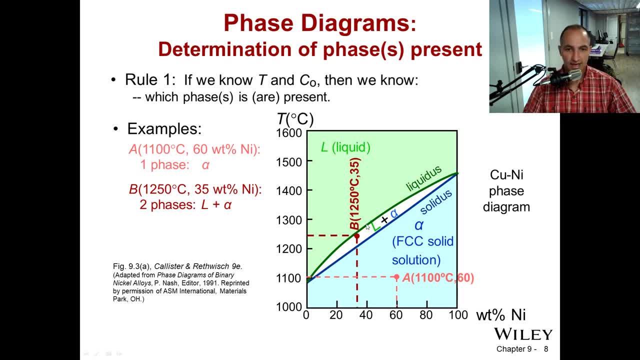 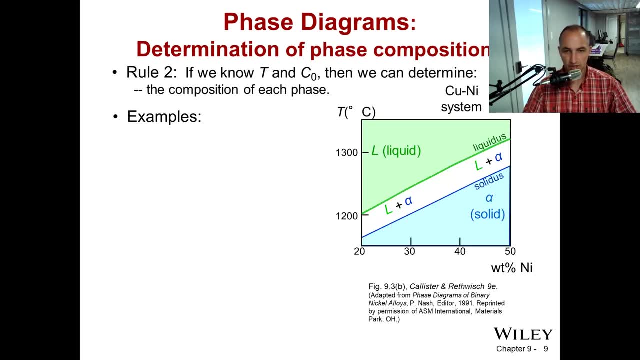 because we're inside this little white area and that is liquid plus alpha. Now we're zooming in a little bit closer in on that area in the phase diagram. So now we're just looking at the region between 20%. Oops, We're looking at the region here. 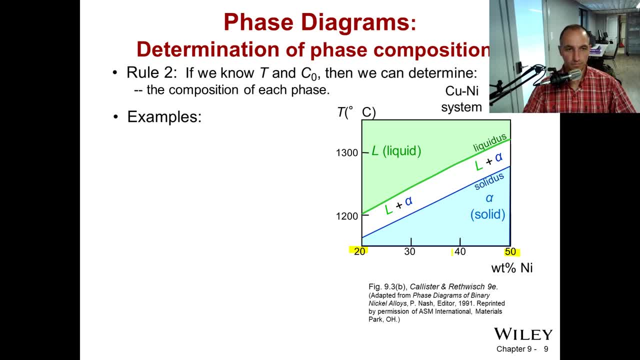 between 20% and 50%. So the second rule: if we know the temperature and the C0, we can determine the composition of each phase. So let's take as an example point A, right here. So the temperature at point A. 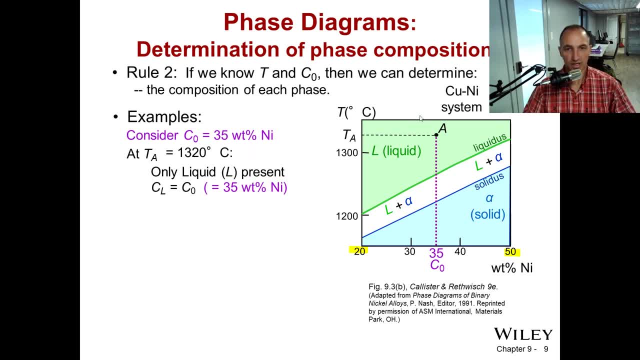 this is given is 1,320 degrees C, and in this area we have only liquid present. So what is the composition of that phase? Well, it's just 35 weight percent nickel, Pretty straightforward: C0,, which is the composition of nickel. 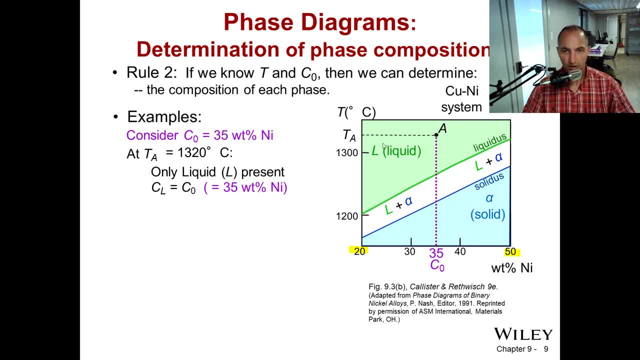 is equal to the overall composition, so that's 35%. Now let's go down here, into the cooler area. here We have 1,190 degrees C, We're all solid and we have only a single phase present, and that is also 35 weight percent. 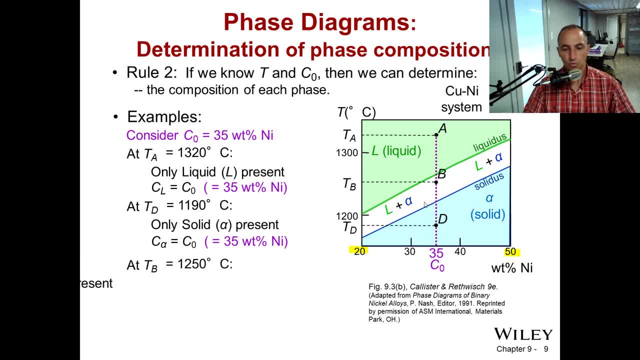 Now it gets a little bit more tricky when we're in the two-phase region at this point B. So in this region we have both liquid and alpha And we're going to draw this black line here which we call the tie line. 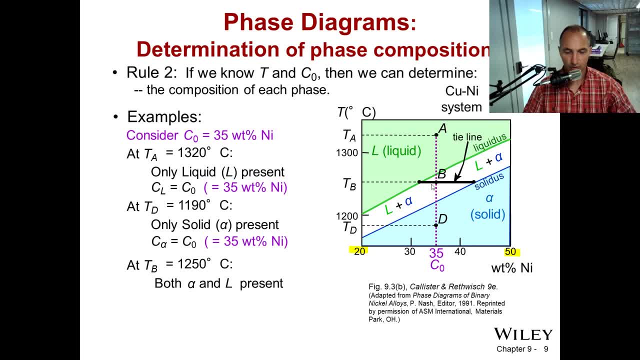 And this is also called an isotherm. We're drawing a line or one temperature and we're seeing where it intersects the edges of that phase region And then we drop down vertically to get composition at that point. So the composition 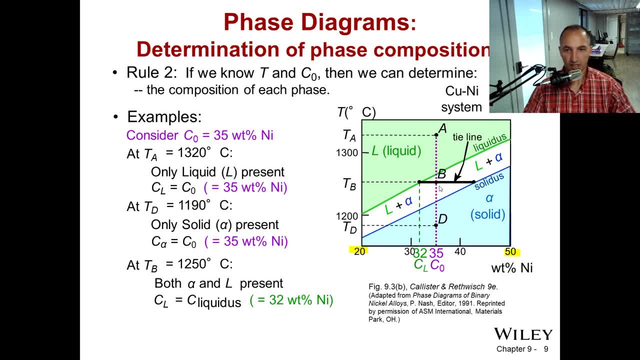 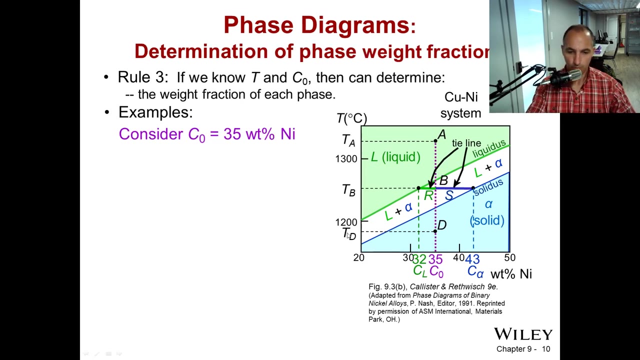 of the liquid, of this slush of liquid plus alpha. the composition of the liquid at that point in time it's 32 percent. The composition of the solid in that slush at that point in time is 43 weight percent nickel. So the third thing we can determine: 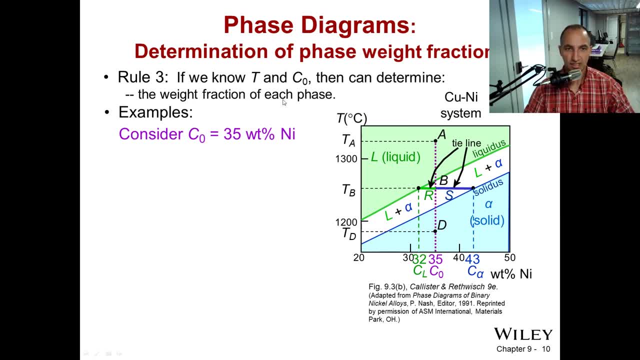 is: what is the weight fraction of each phase? Again, we know the temperature and the overall composition. we can get the weight fraction of each phase. So here we still use the tie line that we had from before And we're still considering. 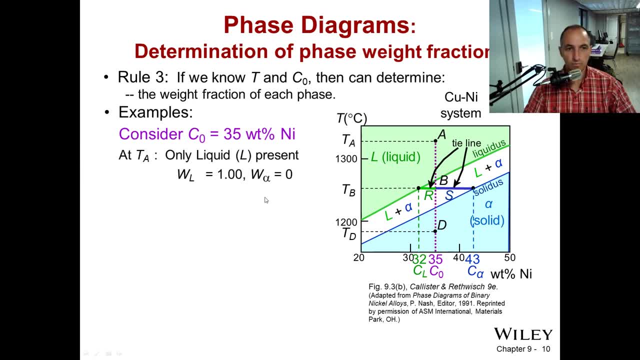 at this 35 overall weight percent nickel At T A. up here we have all liquid. So our weight, our weight percent liquid is one. So we have 100 percent of liquid up here And we have 0 percent of alpha. 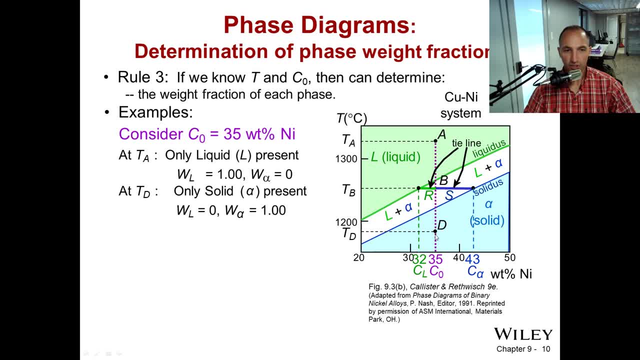 At point D we have 0 weight percent liquid and 100 weight percent of alpha. So we have all alpha at that point, Pretty straightforward. Now in this two-phase region at B we have to do a little bit of a ratio calculation here. 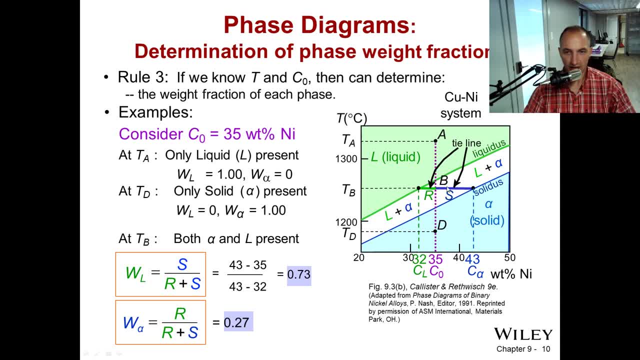 So S is just the length of the line, of the tie line between the solidus and the overall composition over the total length of the line, which is R plus S, And then, if we just pluck those numbers off, we have the 43 minus 34,. 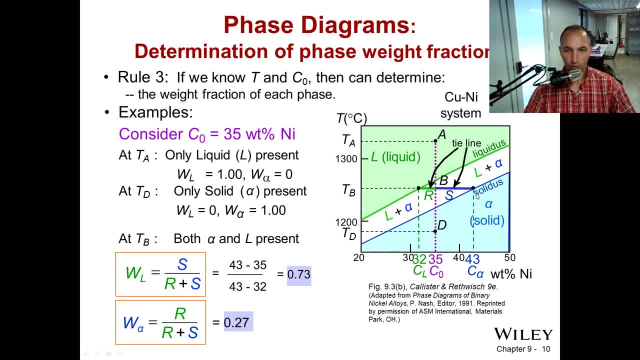 minus 35, over 43 minus 32.. And that gives us a weight percent liquid of 0.73, or 73 volume percent or, I'm sorry, weight percent of liquid. And then the weight percent of alpha is R over R plus S. 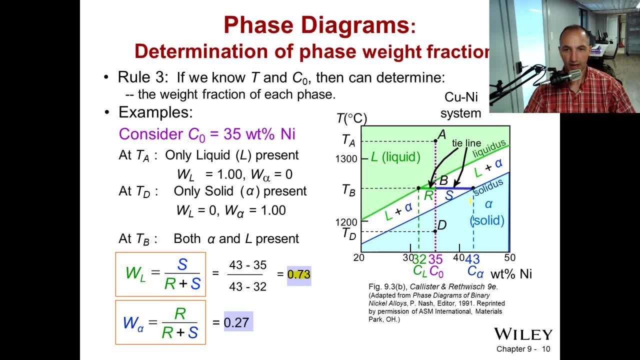 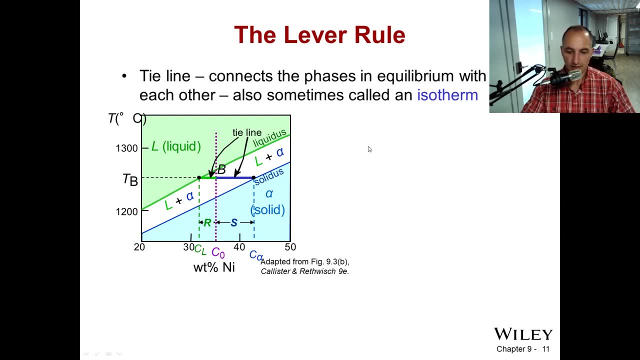 So it's the length of the line opposite of the solid or liquid or phase. I should say that you're trying to determine Opposite. So the tie line. this is called the lever rule, by the way, the tie line represents. 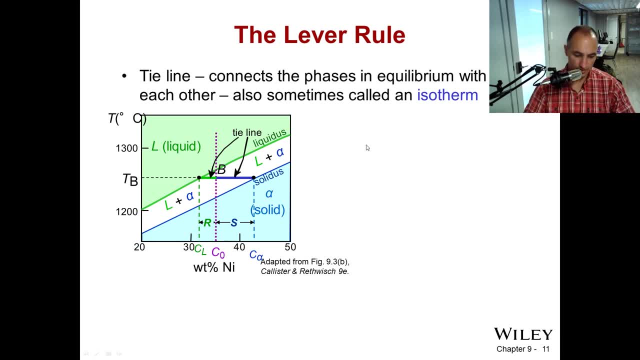 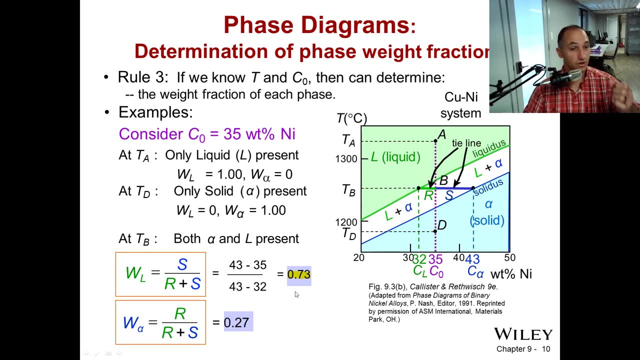 oh, actually just back on that last one there. let's just do a reality check on that, That calculation here. So the weight percent liquid is 0.73.. Does that make sense? Because if you look at this point here, 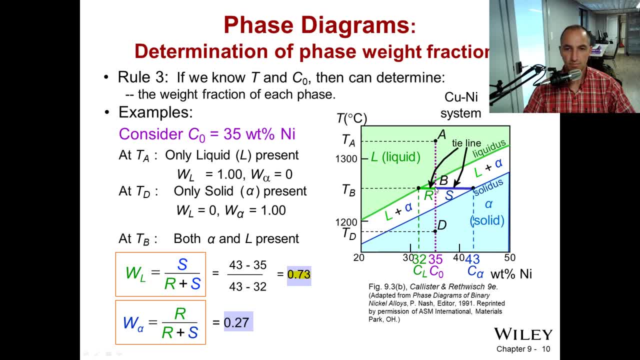 we're only about 25% of the way through the cooling into this two-phase region. So that probably means that we're only going to have- we're going to have- less alpha and more liquid, And as you cool then we're going to get more alpha. 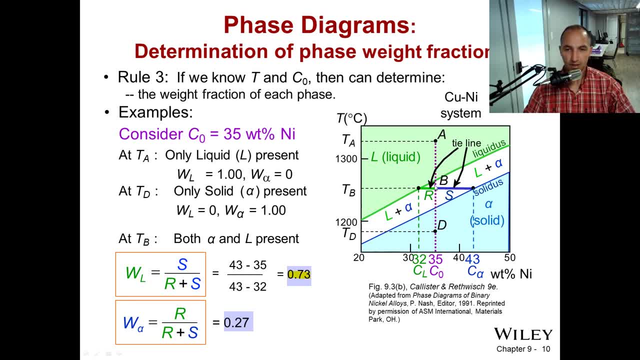 and less liquid. But since we're up here near the top of the two-phase region, we have more liquid, And that's why the liquid is at 0.73 and the weight percent of the alpha is only 0.27.. All right. 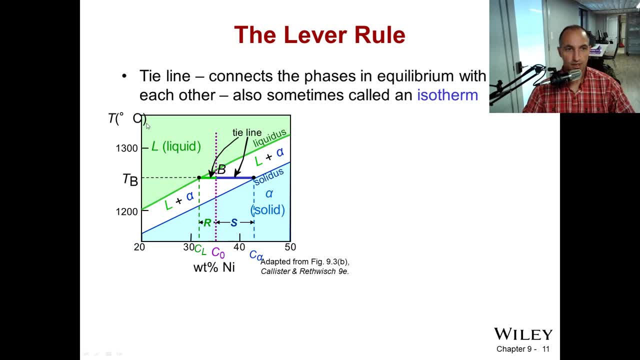 That's a reality check. It's always good to do those when you're working on these problems. So the tie line connects the phases in the equilibrium with each other, And it's also sometimes called the isotherm. So this is your tie line. 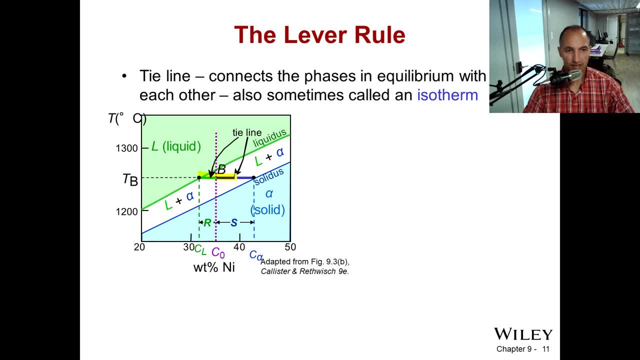 Tie line right across here like this, All right, So what's the weight fraction of each phase? Think of this as a teeter-totter. So if, if you're closer to the top of this two-phase region here, going to have a longer. 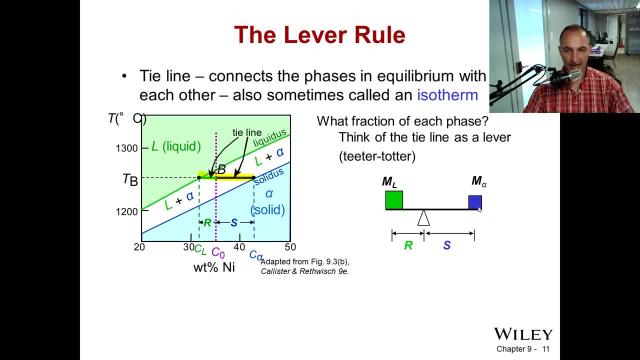 lever on this side, which means that the mass of alpha- you want to keep this in balance- The mass of alpha is going to be smaller, since it has a longer arm, And so that is the length s in this case. So, in order to keep this thing in balance, 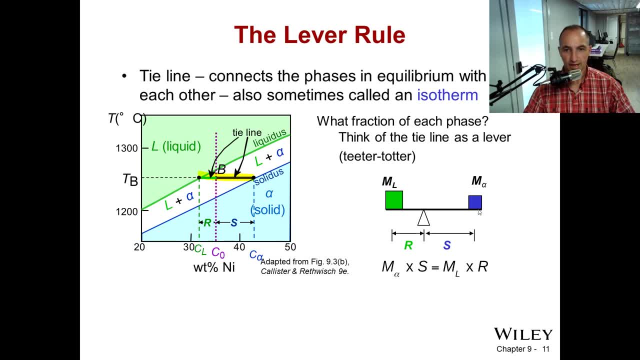 then the mass of alpha times the length of it is equal to the mass of the liquid times the length on the liquid side. So that's r. So to keep that in balance, that's how it works. So the weight percent of the liquid: 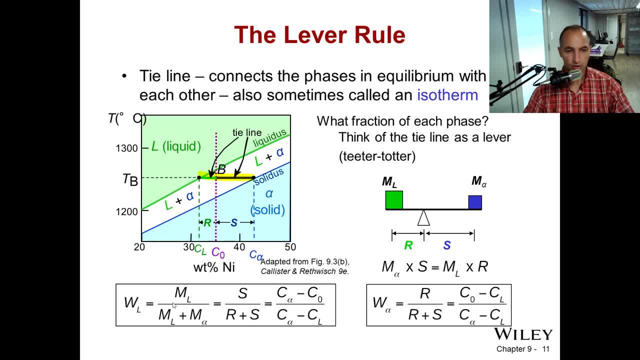 is just the mass of the liquid over the mass of the liquid plus the mass of the alpha, And that's equal to s over r plus s, Or the composition of the alpha minus the overall composition over the composition of alpha minus the composition of the liquid. 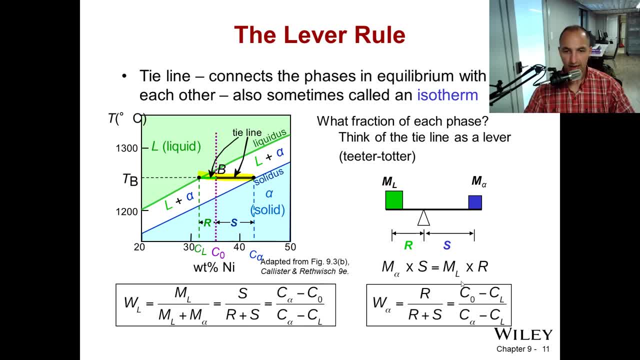 That's the total length of the tie line. And again for the weight percent of the alpha, just take the length of the tie line opposite of alpha from alpha over the total length of the tie line And you don't have to do both of these calculations. 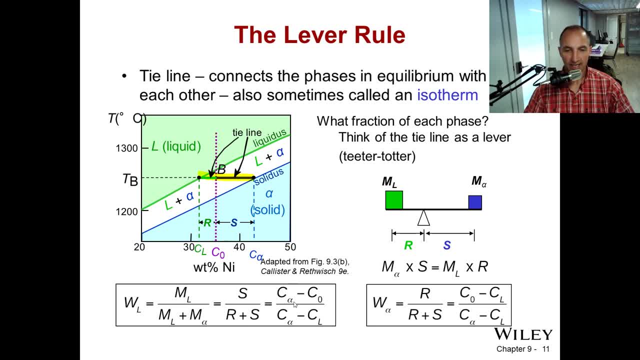 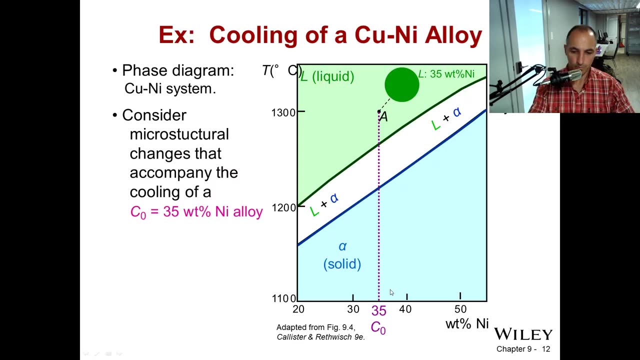 because once you calculate one to get the other one, since this is a binary base, the other one is just one minus the other one. So just pick one to do and then easily calculate the one after it. So let's look at cooling. 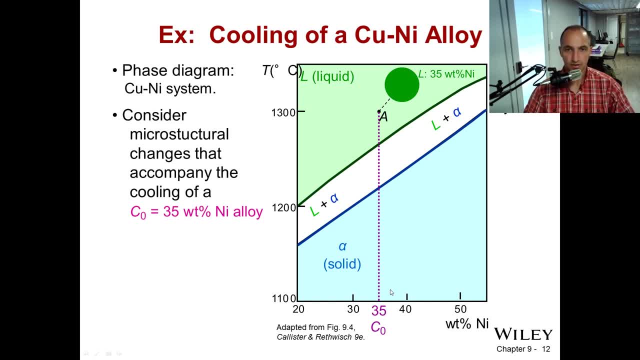 of this copper nickel alloy and look at the microstructure changes that are that accompany this cooling. So, starting out again, we're at 35 weight percent nickel and we're at a high temperature here of about 1300.. We're going to have all liquid. 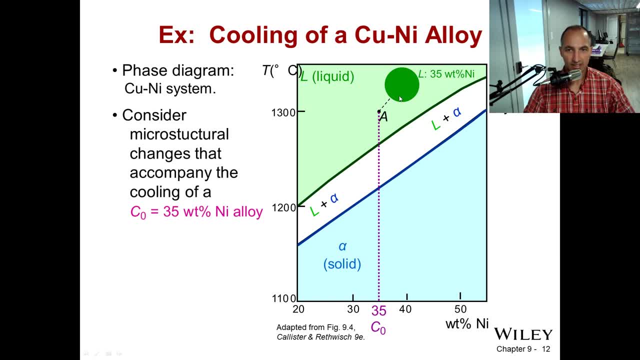 And the weight percent of the nickel in that liquid is at 35 percent At b. just start to precipitate out some solid of alpha In there And the composition of those little alpha precipitates are going to be 46 percent And the surrounding liquid 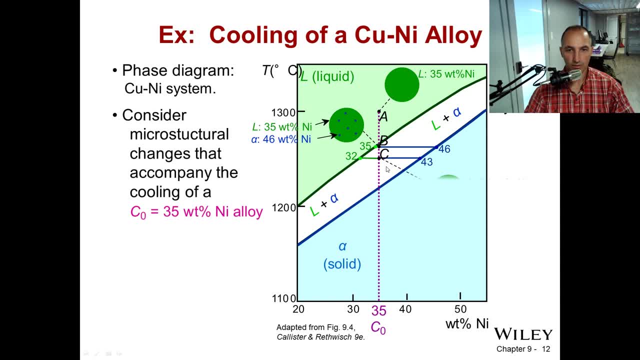 is still at 35 percent And as we continue to cool, now the alpha composition of the alpha starts to decrease because we're going down this tie line here, Going down this tie line. So now the solubility of nickel and alpha. 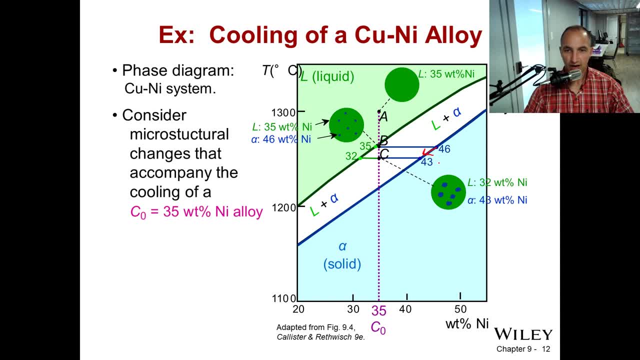 starts to decrease. So now our alpha composition is only 43 percent And our surrounding nickel is at 32 percent. And now we're cooling further. Our alpha is now all at 36 percent And the liquid composition is at 24 percent. 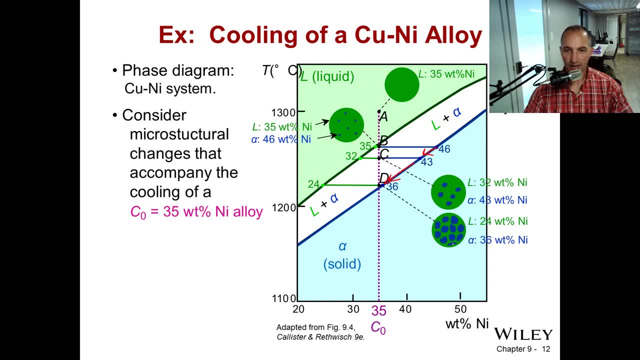 Now we have much more alpha and a lot less of the liquid. Now at e, all the liquid has been converted into solid and we have 100 percent alpha and the composition of the alpha is 35 percent. So it's the same as the overall composition. 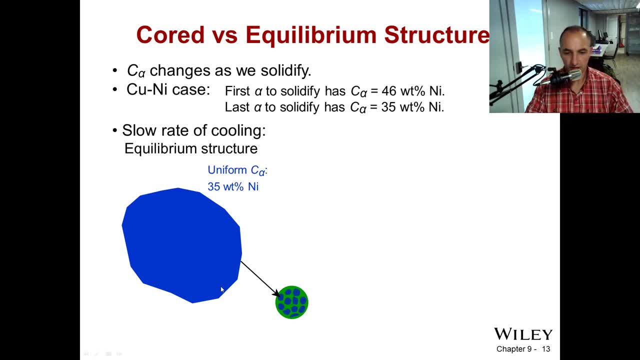 So what you saw previously was equilibrium cooling, And whenever you hear the word equilibrium in thermodynamics, you have to think: painfully slow, ever so slow. everything is happening, But in reality that's not what happens In this case, what really happens here. 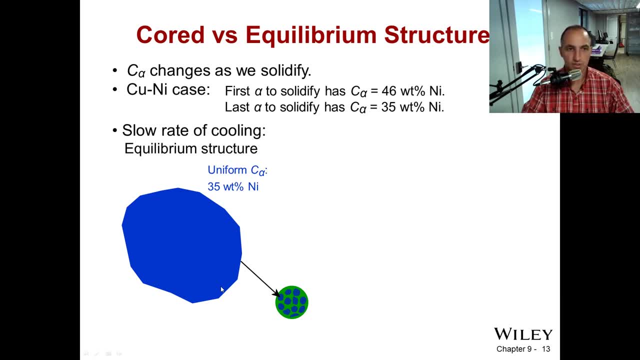 you have something called coring. So the composition of alpha is changing as we solidify. The first alpha to solidify had 46 weight percent. As you continue to solidify it keeps dropping. Eventually it reached 35 percent. So what happened to all that nickel? 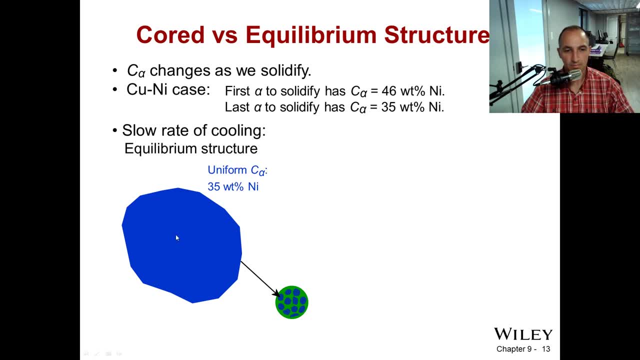 that had first solidified Well what happened, because this is painfully slow. there was enough time for the nickel that was in the center of here to diffuse out and get ejected into the liquid around it, But in reality we have faster cooling rates. 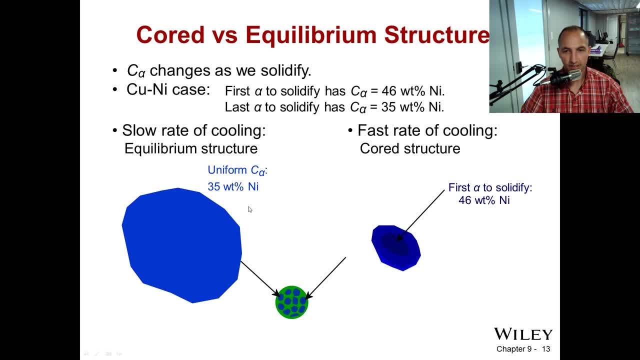 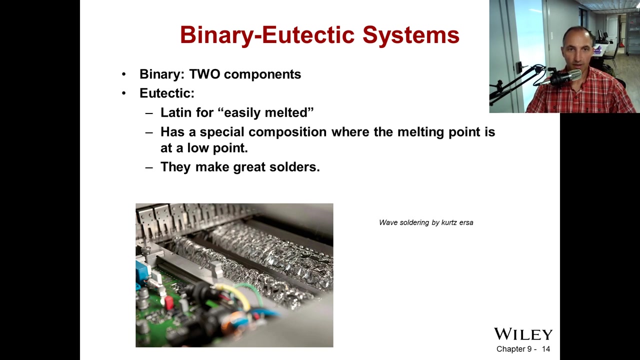 than we thought. So the first nickel is at 46, then it goes lower and lower, lower, and the last alpha to solidify is less than 35 weight percent nickel. Alright, moving on The binary eutectic system. 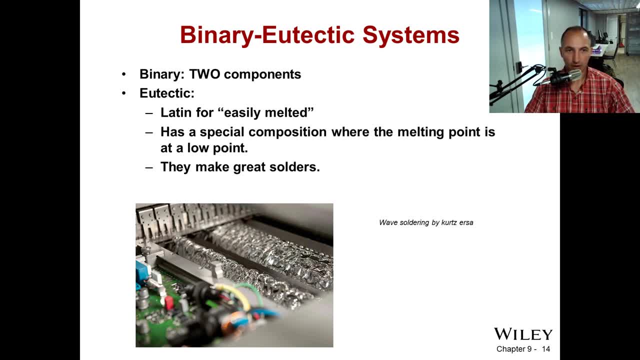 means two components. We're still on two components And we're now talking about eutectic systems. So eutectic is Latin for easily melting. So a good example of a special composition is solder, And there is a silver tin. 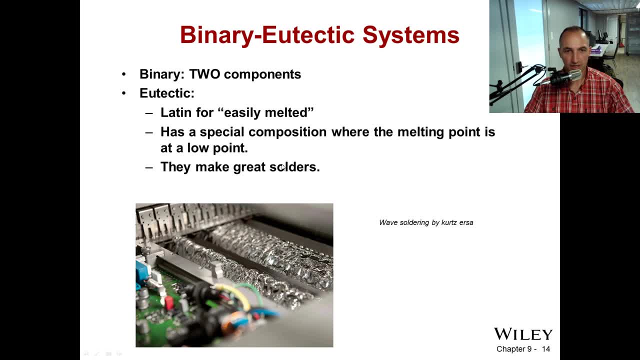 or there's a composition where the melting temperature is at the very lowest And that's a special composition and it only occurs at one composition. So that's why they make great solders, because we can use them without having to heat them up very much. 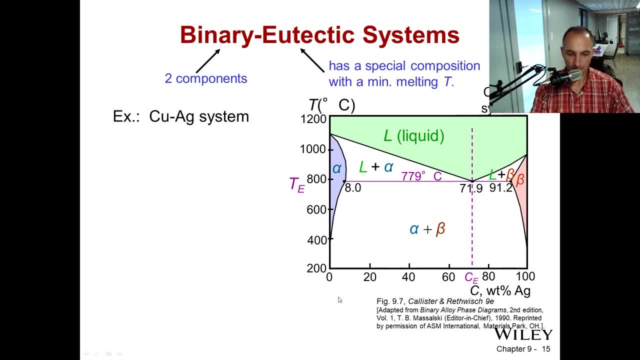 So binary means eutectic. Remember, easily melting. Eutectic means easily melting. It has a special composition with a minimum melting temperature And this purple line right here is eutectic composition And it has a melting temperature. 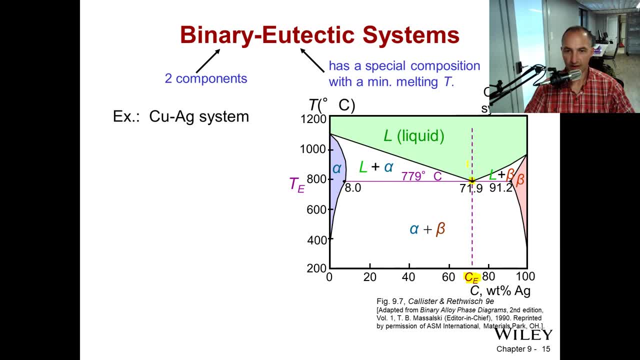 of only about 800 degrees C right here And there are three single phase regions. We have either all liquid and then we have alpha plus beta down below, And no matter where you are in this phase diagram, you're going to have only three phases. 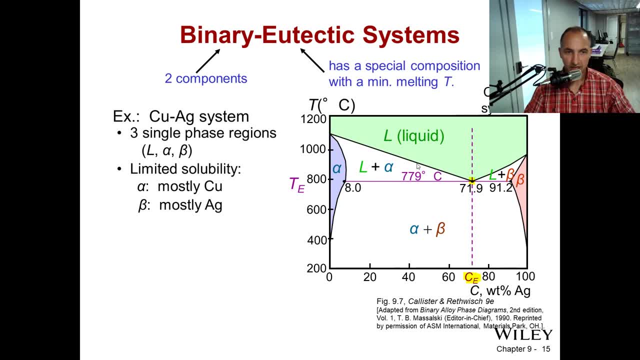 possible And there's a limited solubility here. It isn't complete solid solubility like we had in the previous example where we had all of the Hume-Rothory rules were met. In this case you don't have all the Hume-Rothory rules. 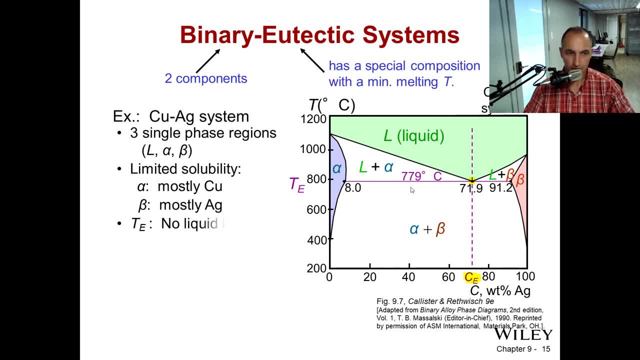 met for this type of system And at the eutectic temperature, which is Te, there's no liquid below Te. That's this horizontal line right here. You never have any liquid below that, no matter what composition you're at, And the 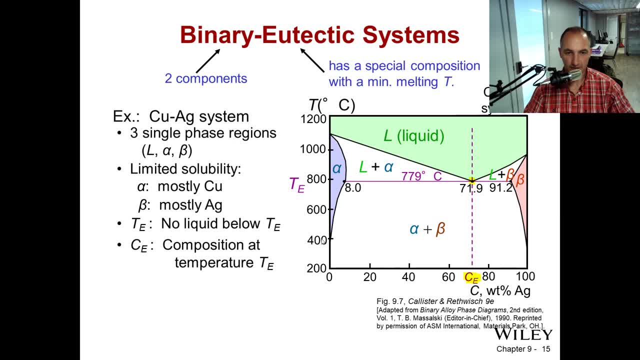 composition at the eutectic temperature is Ce. The eutectic reaction at this composition, which is at 71.9 weight percent, silver is all liquid going to alpha plus beta, And so that is actually 71.9 weight percent. 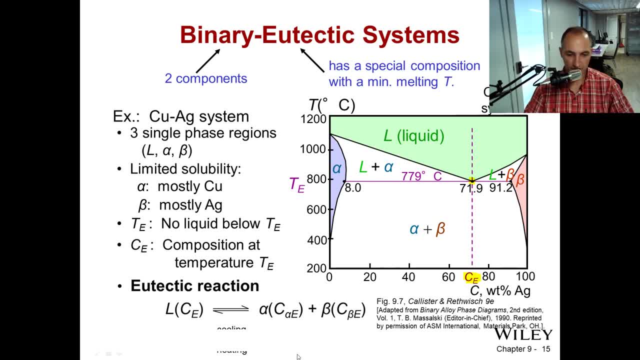 silver going to alpha, which is eight weight percent. right here, eight weight percent alpha and 91.2 weight percent of the eutectic temperature at the eutectic temperature, at the eutectic temperature of silver in beta. So the 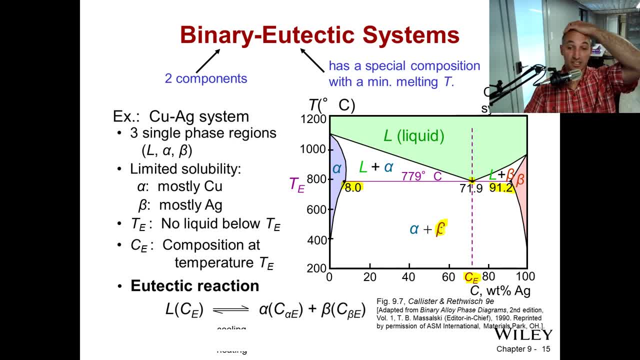 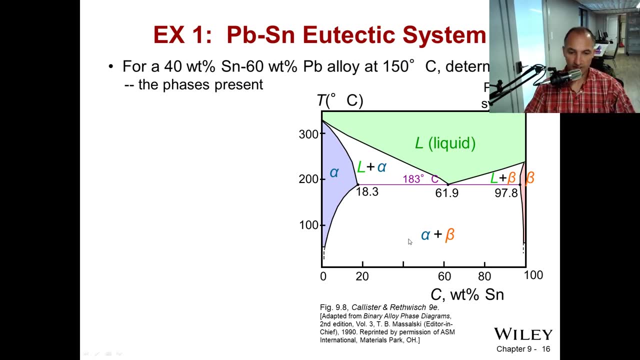 beta here is going to be very rich in silver and the alpha is going to be very rich in copper. Let's take this example, let's look at this, and let's look at this example. let's take this example, let's make this. 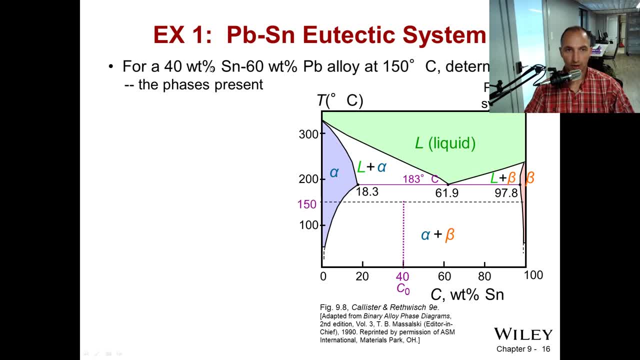 example, this is: this is a split lead, and the first question of the multiple lead we're going to ask is what phases are present? well, at 150 degrees C, guess what? the answer is alpha plus beta. so that's the answer to that question. now, second question: what are the compositions of each of the phases? so 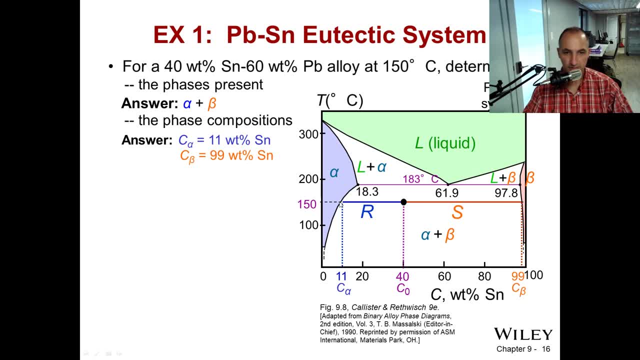 let's draw that isotherm where it intercepts the alpha and then drop down to the composition and there we have 11% of 11% tin in the alpha and you have 99. you have 99% over here. you have 99% of the tin in the beta. 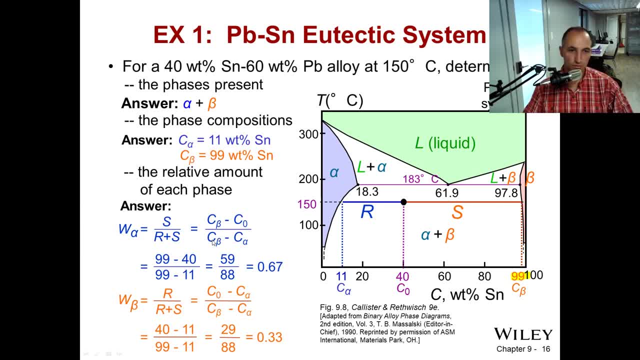 the last question to answer. what is the relative amount of each phase? this is the weight percent of each phase, so let's use this tie line. here we're going to be looking at the length of the line which is s, length of the line which is s. 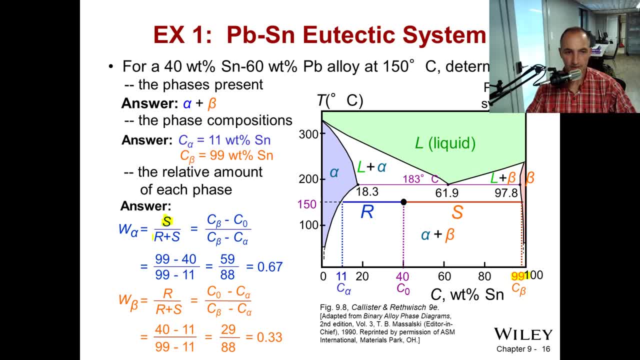 over the total length, R plus S, R plus S. so that is just the composition of beta minus the overall composition over the composition of beta, minus the composition of alpha, and plugging in those numbers, 99 minus 40, 99 minus 11, get 0.67. so that's 67. weight percent is going to be alpha at this. 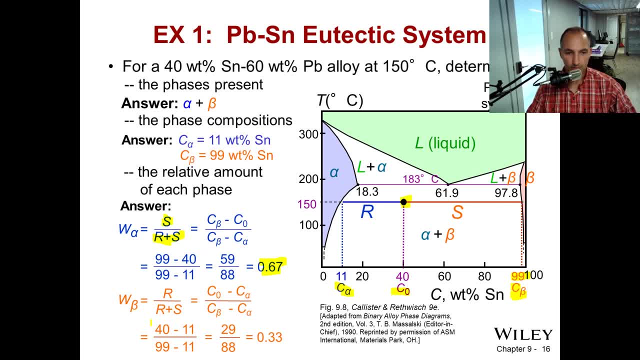 point right here. now the weight percent of beta is the length of R over R plus S, R plus S here and plugging in that, so that would just be overall composition minus alpha, composition all over composition of beta minus composition of alpha, and that equals 0.33. 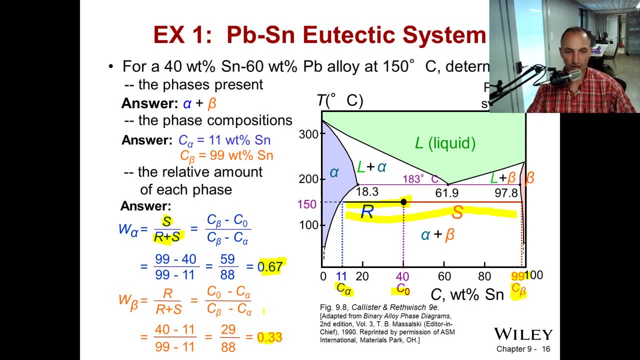 the notice here is, as I said earlier, you only have to calculate one of these two, so that weight percent of beta could just be one minus 0.67. one minus 0.67 is 0.33, and that's how we're going to do it later on. we're going to do that. 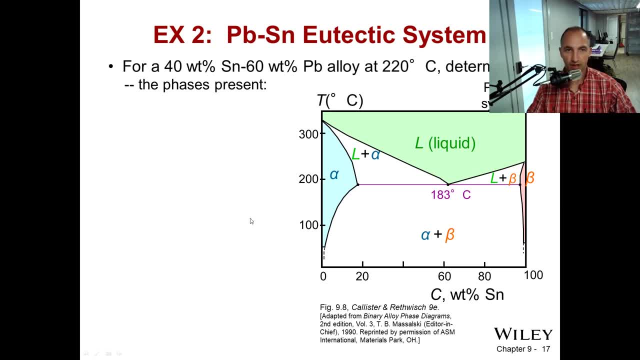 little shortcut, let's look at another example of the same system, of the lead tin eutectic system, and we're going to look at the same composition of 40- 60, but we're going to go to a higher temperature of 220 degrees C. so 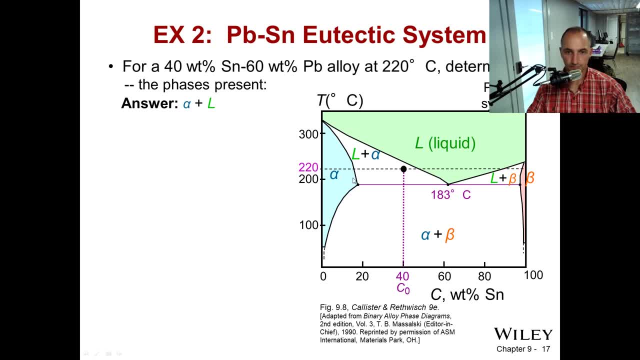 let's draw a horizontal line 220. we have what we have: two phases here, alpha plus a liquid. so we're in like the slushy here region and we're below the eutectic temperature, I'm sorry, the eutectic composition. second question: 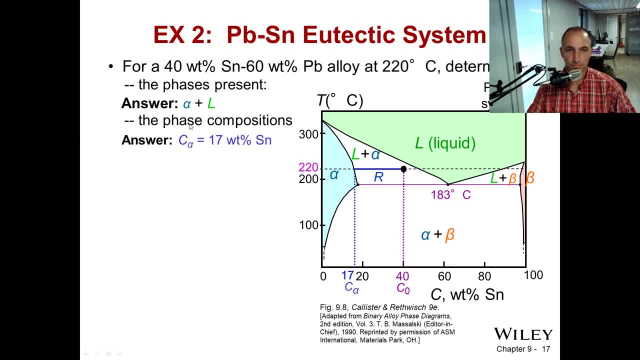 what are the compositions of each phase? these compositions draw that horizontal isotherm until it intercepts the. the next phase that it comes across here is alpha. so that means 17 weight percent of tin is in that alpha phase and 46 weight percent tin is in the. 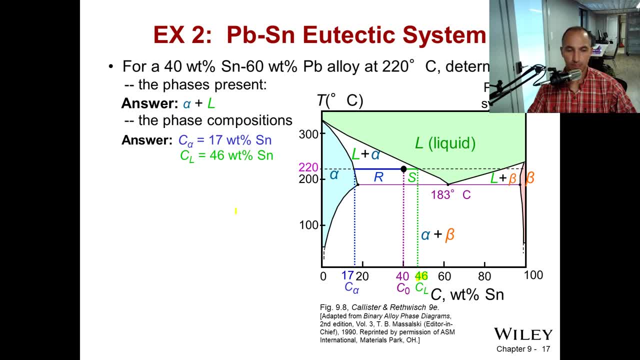 46 weight percent. 10 is in the liquid. now let's look at the relative amount of each phase, the weight percent of each phase. so that again is the length of. so for alpha, which is on the left side here, so we have to go to the opposite line. so that means that that's the length which 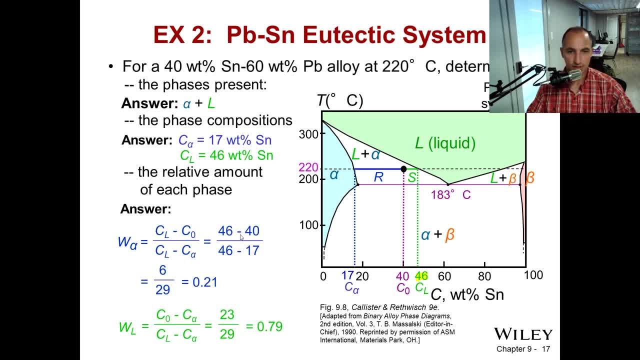 is s over r plus s. so 46 minus 40, 46 minus 17, that gives us 0.21 weight percent alpha. so the weight percent of the liquid is just the line that's opposite the liquid. so that's r over r plus s. 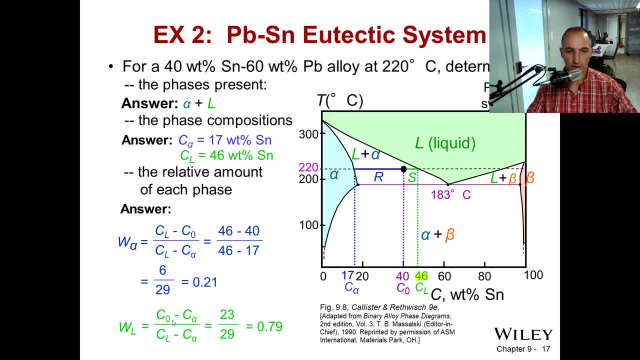 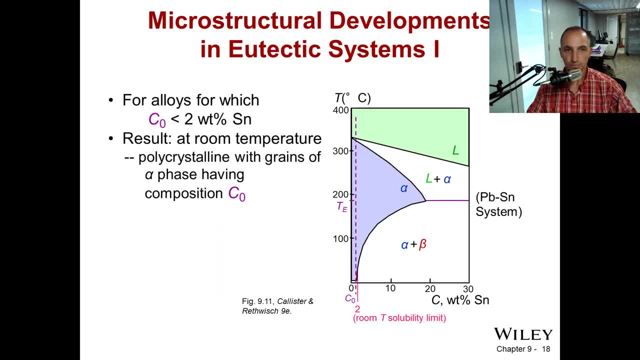 we've answered all three questions, for example two. so the microstructural developments. we're going to look at the microstructural developments in eutectic system. we're going to start out looking at a very, very small weight, percent of tin but room temperature you have polycrystalline with grains of alpha. 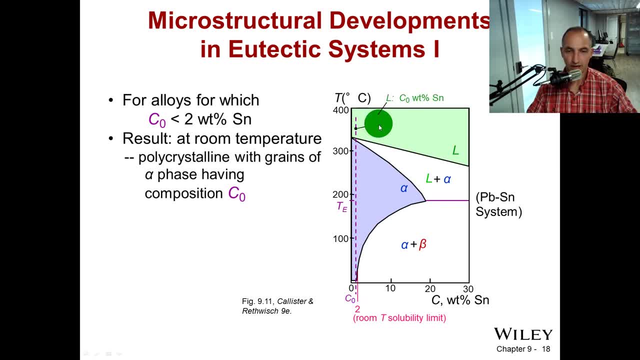 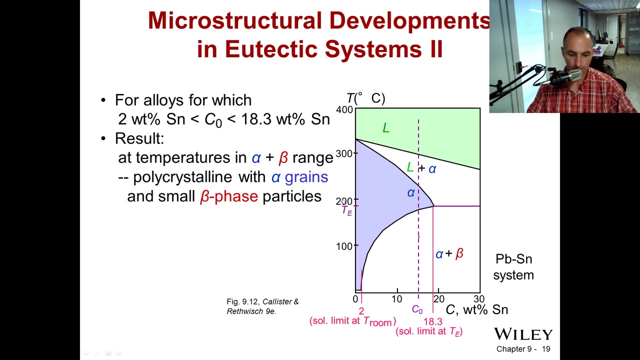 phase. here we start out with 100% of liquid and as we cool, we start to get some alpha. cool further, we form all alpha, all alpha, and the composition of that alpha is just C0, the overall composition. now let's go to a higher composition of 10. so let's look at what happens between eighteen point. 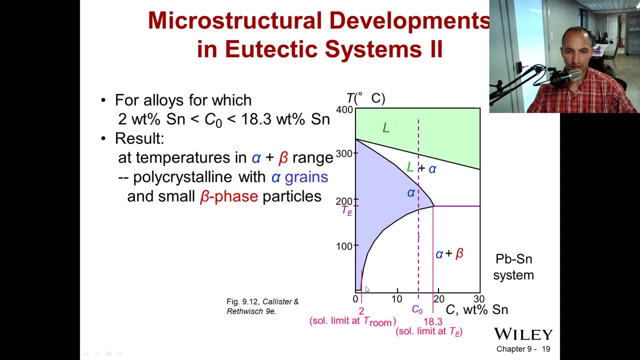 three percent and two percent. so that's this area between these two red lines. here they're looking at this red line, this red line, so all this area in between here. and so the result: here again we're all liquid cooling. we're getting alpha solid particles forming in this slushy of liquid. now all of the 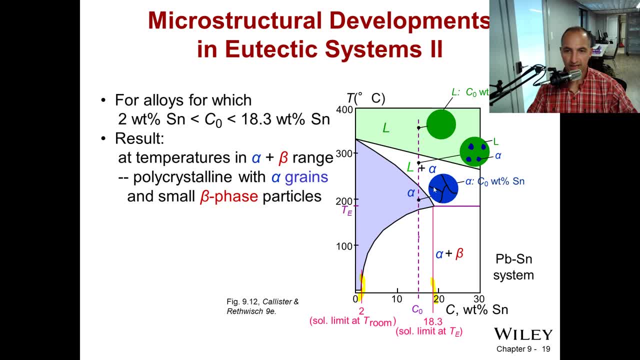 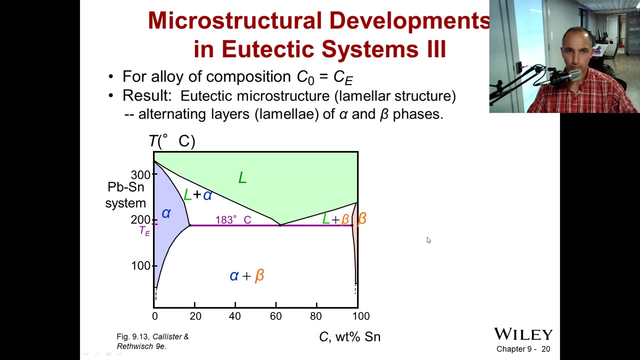 alpha has converted and it's still just the overall composition of 10, and now we have these little tiny precipitates of beta in the alpha. so that's what the microstructure will look like in this area here all right. now let's look to see what happens when you're when you're at the 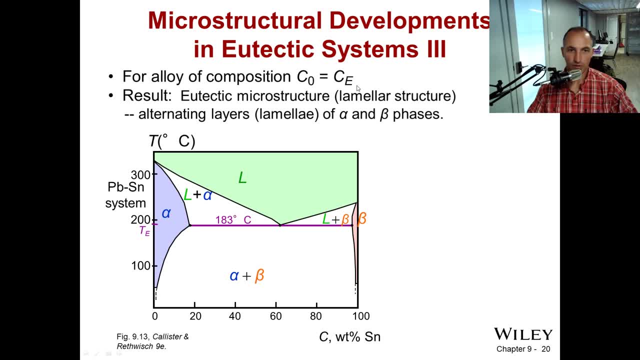 eutectic composition. the eutectic microstructure is lamellar and is a lamellar structure, a lamellar, the lamellar structure. so the eutectic composition is 61.9%. starting out all liquid at high temp and then immediately, without any partial solidification. it solidifies quickly. 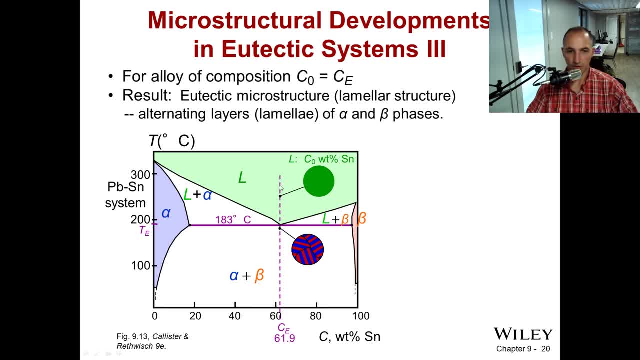 to alpha plus beta. this is a. this is a great way to work with solder. you don't have to worry about partial cooling it. it will just cool and solidify very quickly, which is exactly what you want in a solder, so that this lamellae is 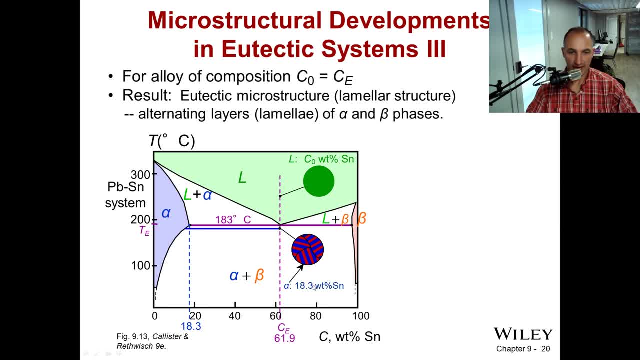 composed of alpha plus beta, and the alpha is blue, beta is red. and what? what is the composition of the alpha and the beta? so the composition of the alpha is just the blue line here. drop that blue line down and you have 18.3% weight. 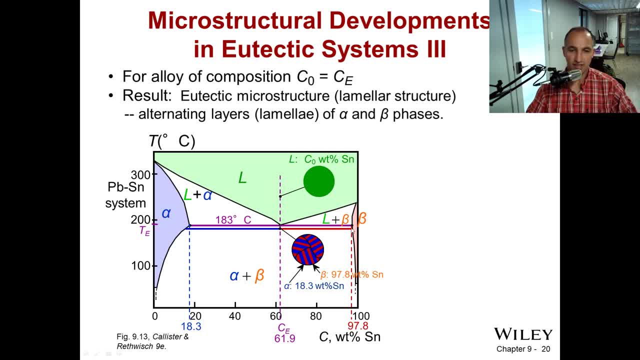 percent, alpha and the weight percent- I'm sorry, not that way- percent, the composition of the beta is ninety seven point eight weight percent, and so it's not completely round and it's not necessarily double-sided, but this is pretty solid. so, and and a micro, the microstructure of what that looks like is here. you have these. 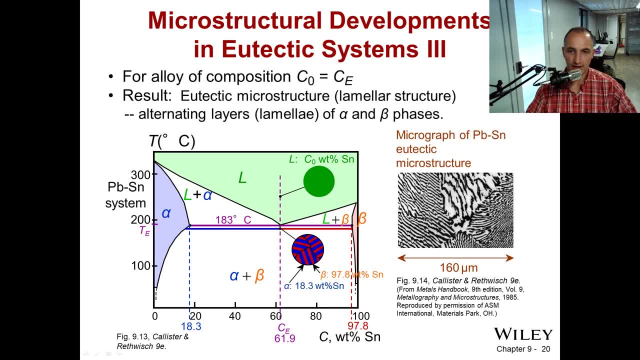 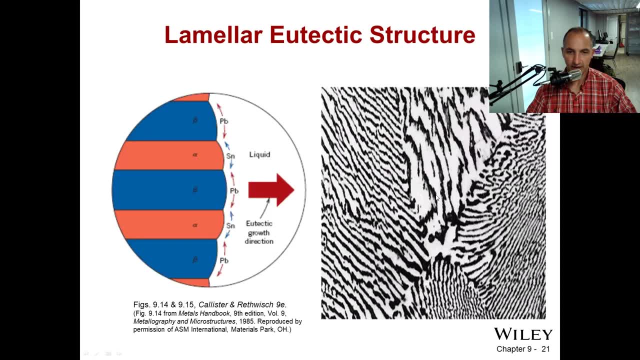 black like zebra stripes, and of alpha and beta. that's eutectic microstructure, so at much smaller scale here, as we see what's happening here: that the lamellae is growing out of the liquid and the beta is tin rich, so it has to eject lead out of it and the alpha here is is lead. 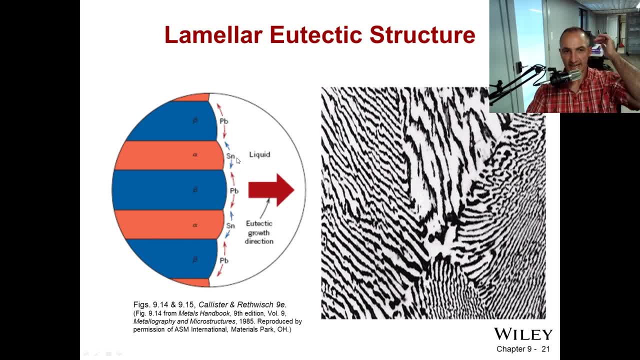 rich, so it has to eject the tin out of it. and the faster the solidification process occurs, the finer these lamellae become, so this thicknesses of these phases become much smaller as you have faster cooling, because there's just not enough time to diffuse the, the lead and the tin. 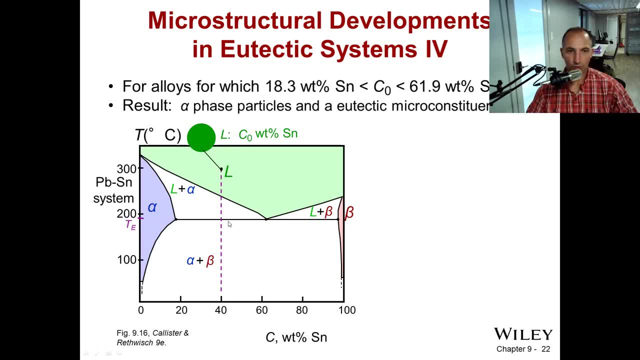 out all right. so let's look at a composition below eutectic composition. so this is for any region between 18.3 and 61.9. so we're looking at anything between here and here. we start out with pure liquid. as we solidify, we start to precipitate out these alpha. 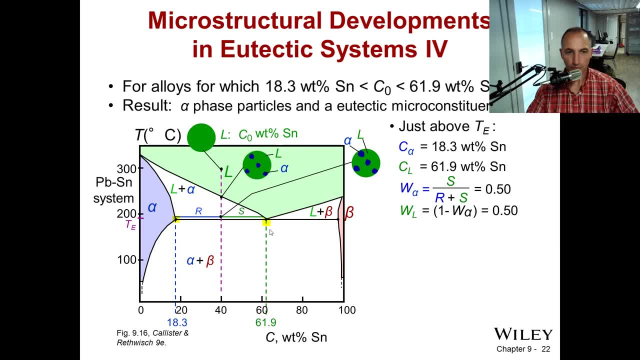 and the alpha get bigger as we cool and just above the eutectic temperature. the composition of the alpha is 18.3 and liquid is 61.9 and the weight percent of the alpha is S over R plus S, and the weight percent of the liquid, which is the green line here, is just 1. 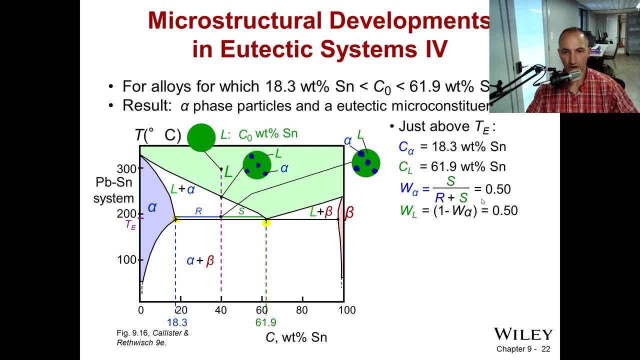 minus that, or you could just do R over R plus S, so it's 50% weight, percent alpha, 50% of the liquid and just below the eutectic temperature. we solidify out all of the remaining liquid into the lamella, and that is since it happens instantaneously. 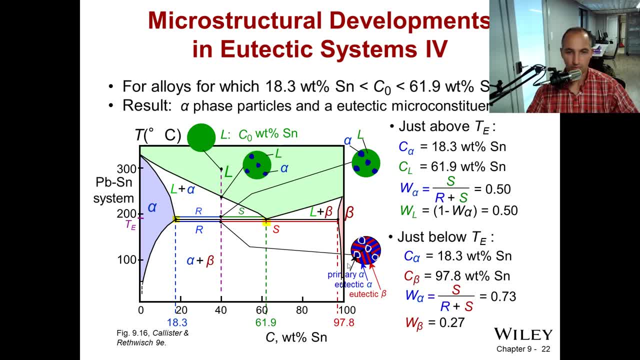 then that's why you don't have any time to form, like you know, large phases of one versus the other. it's this lamella phase that forms, so we call this primary alpha, which are these, you know, blue blobs here. that's the primary alpha, and the eutectic alpha is these blue lines in the lamella. 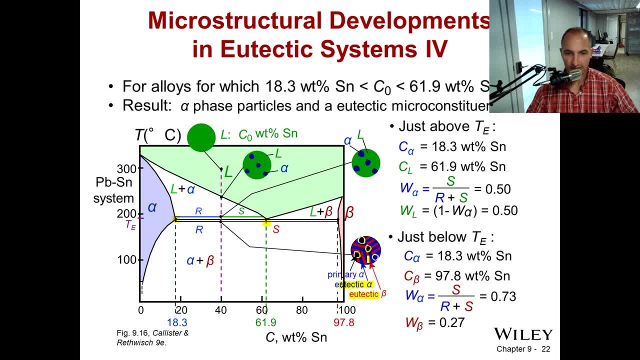 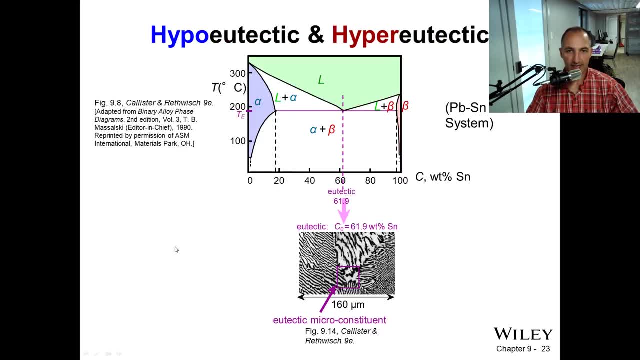 and the eutectic beta is the red lines in the lamella. so hypo-eutectic and hyper-eutectic- I'd like to introduce these terms to you now- where hypo is any composition below the eutectic composition. but so in anything in this region is hypo-eutectic and this region is hyper-eutectic. 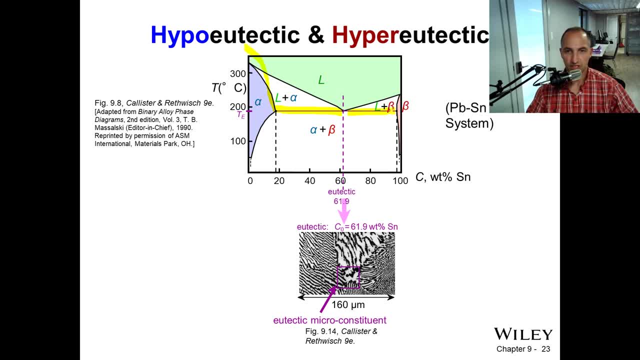 hypo and anything in this region here is hyper. so the hypo eutectic: we were to cool anything down through here. we're going to have primary alpha particles and then we're going to get the lamellae at the below the eutectic temperature. so this here is the hypo eutectic, the hyper. 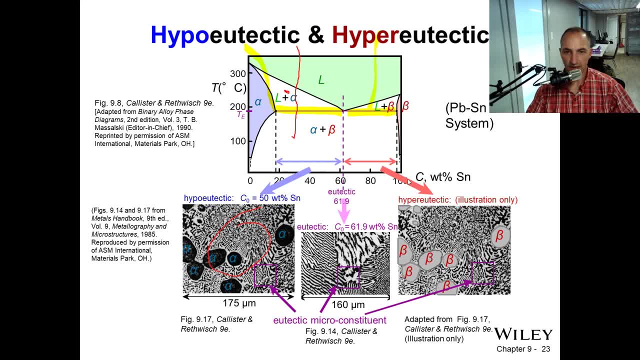 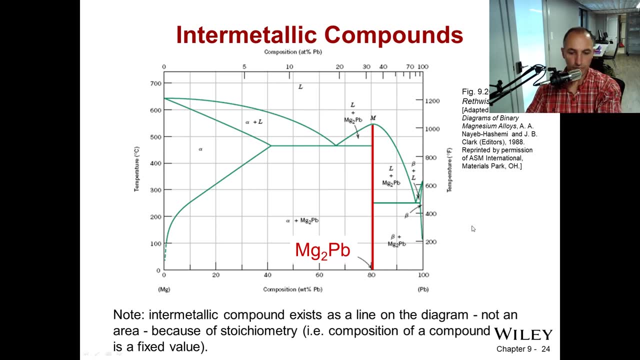 eutectic. now we have primary of beta and we have eutectic alpha plus beta. so that's the hyper eutectic. you now. this phase diagram is a little bit more confusing, but I'm bringing it up because I want to introduce a few more terms here, which are the intermetallic: 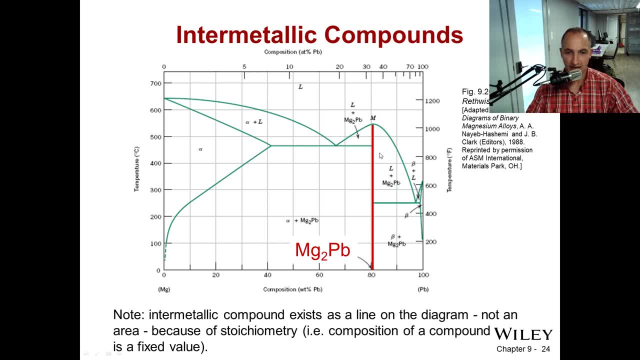 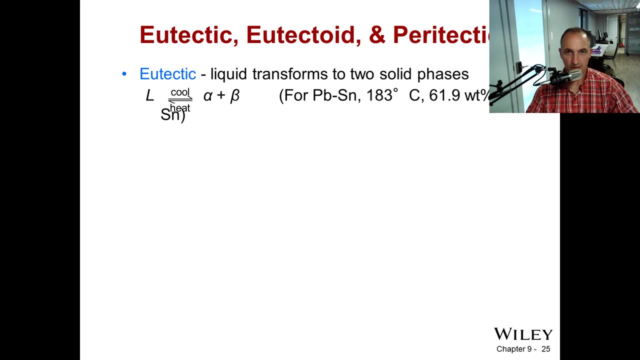 compounds. intermetallic compounds exist as a line on the diagram, not as an area. this is because they're stoichiometric, ie the composition of the compound is a fixed value. all right, so eutectic, eutectoid and peritectic. we talked about eutectic, this. 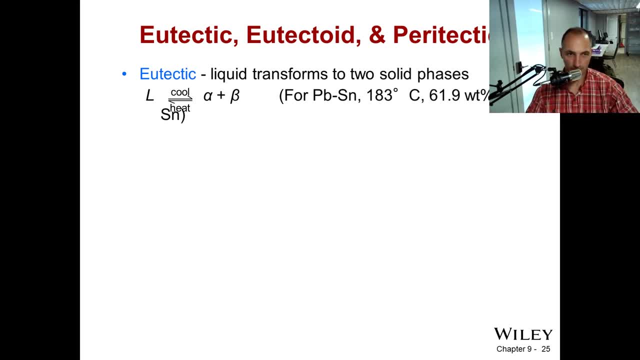 is liquid cooling to form alpha plus beta and brought up the example of lead tin at sixty one point nine percent. ectoid is a new term here, and this is very similar, except instead of cooling from a liquid to two solvents, this is a liquid cooling to form alpha plus beta, and this is very similar, except instead of cooling from a liquid to two solvents. 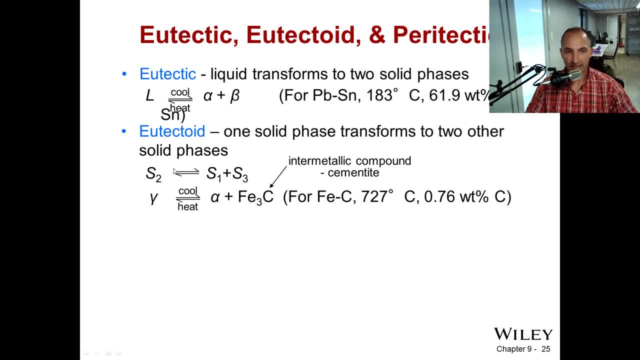 we already have a solid and we're taking that solid and we're breaking it up into two separate solid phases. an example of this, which I haven't shown you any phase diagrams yet, for this is just gamma cools to alpha plus iron carbide, and this occurs at point seven, six weight percent copper. I'll show you some. 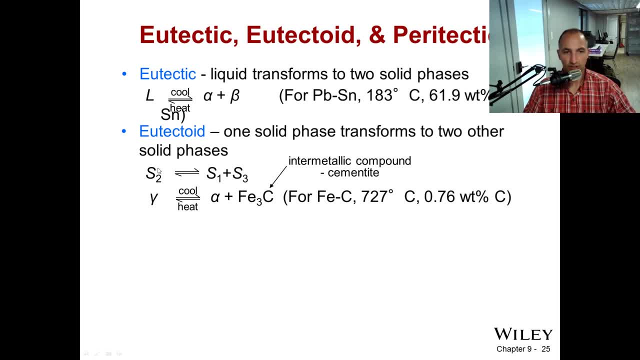 examples of that later. so that's eutectoid, which is a solid, and going to two other solids. a peritectic is a liquid and one solid phase transforming to a second solid phase. again. we see this in the iron- iron carbide phase diagram, where you have a solid plus a liquid going to a solid. 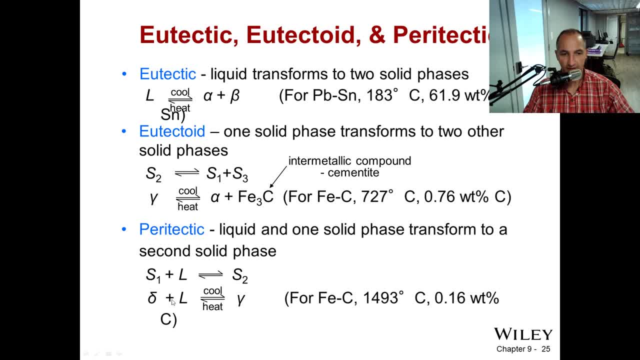 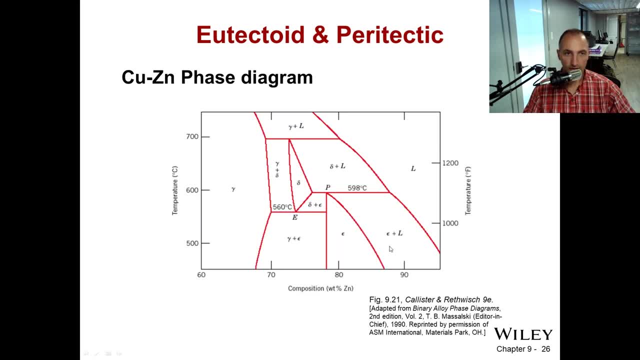 example, here is the delta iron plus liquid going to gamma iron. here's the copper zinc phase diagram and I'm going to point out a eutectoid transformation here and this is just a delta phase. the delta phase here cooling down through here to a gamma plus epsilon. 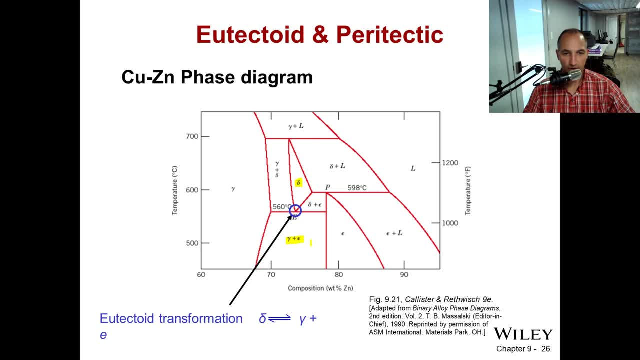 phase. so that's eutectoid: one solid going to two other solids. a peritectic transformation is a peritectic phase. so here we have two solids, gamma plus- I'm sorry- a solid plus a liquid going to a single solid going down here to Delta. so that's a peritectic transformation. 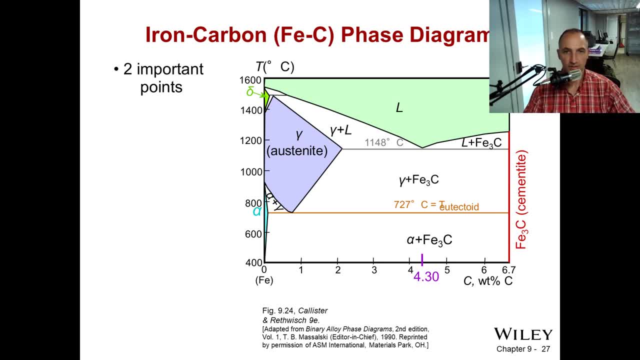 okay, so let's look at the iron carbon. I promised you this: looking at the iron carbon phase diagram. there's two important points in this phase diagram. oh and FYI this: the composition in this phase diagram only goes up to six point seven weight percent carbon. it does not. 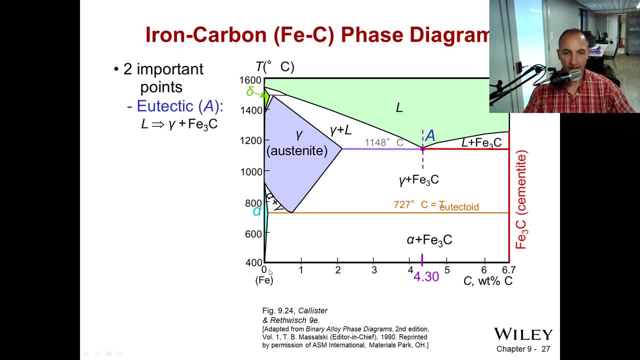 go all the way up to a hundred percent, and that's because the rest of the phase diagram is not useful to us and we've always just focused on this area of the phase diagram, the two important points. you have the eutectic at alpha liquid going to two solids. this is liquid going to gamma iron plus iron. 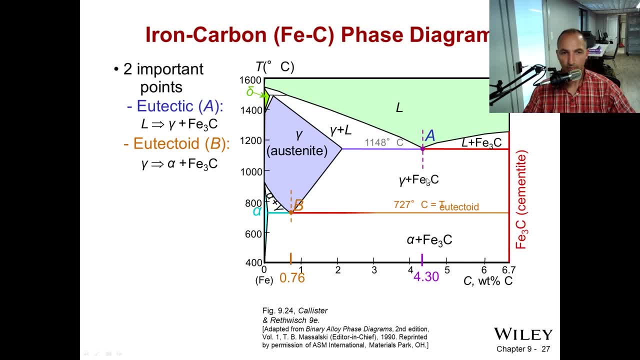 carbide and the eutectoid solid going to two other solids is gamma. we also call this austenite. by the way, you have austenite going to alpha plus iron carbide. alpha is also called ferrite. the iron carbon phase diagram you have. 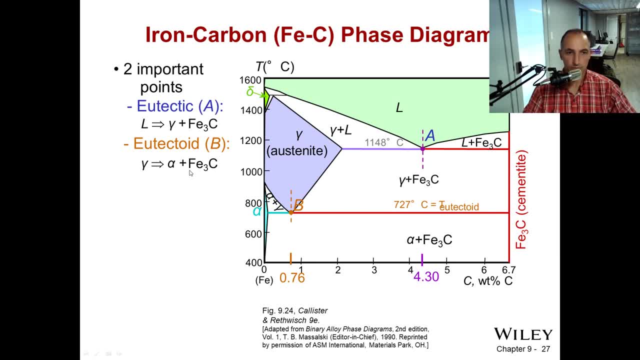 alpha plus iron carbide, that's eutectoid and the. because we're going through a you, this horizontal line here. it's going to form that lamella. so anytime there's eutectic or eutectoid, you're going to get the lamella structure always okay. so that is what the 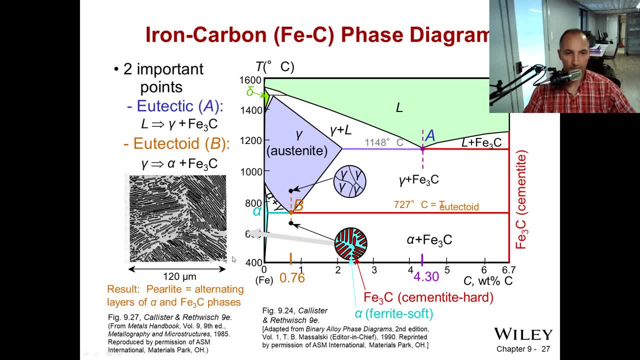 you microstructure will look like. and that lamellite- we give it a special name in the iron carbon phase diagram and we call that pearlite because it looks like, I guess, mother of pearl when you look at it under a polished sample looks very beautiful. so those, these are just alternating layers of alpha plus. 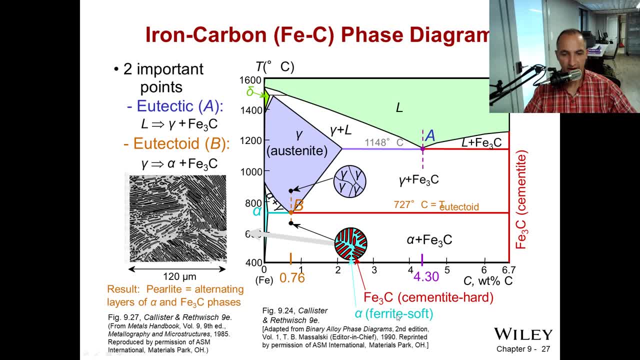 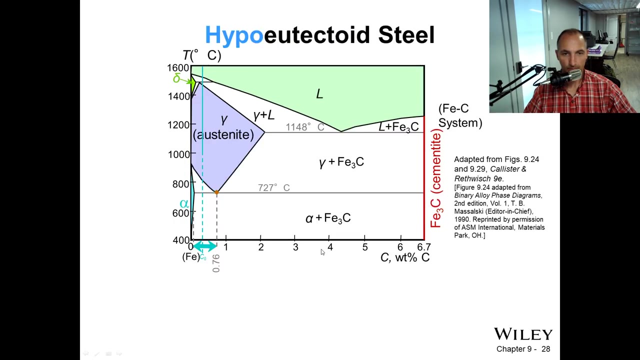 iron carbide alpha is called ferrite, that's soft and you. it's soft because it has a low carbon content, and the cementite, which is fe3c or iron carbide, that's very hard. so the combination of those two is called pearlite hypo. eutectoid steel hypo, as you remember, is below the eutectic composition and 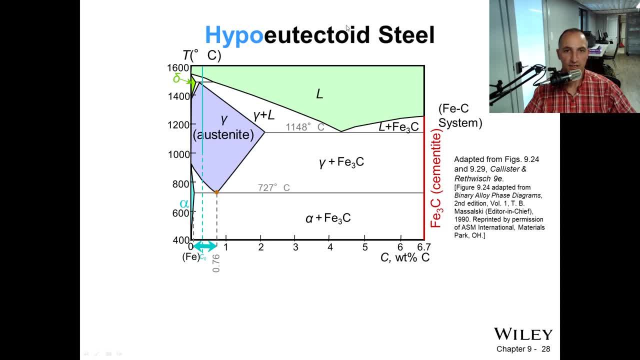 and it's oid meaning solid- going to two other solids. so, looking at the cooling of this austenite or gamma iron, it's all austenite and start forming precipitates of what you start forming, precipitates of alpha right in this area and then that alpha starts to consume more and more of the austenite. 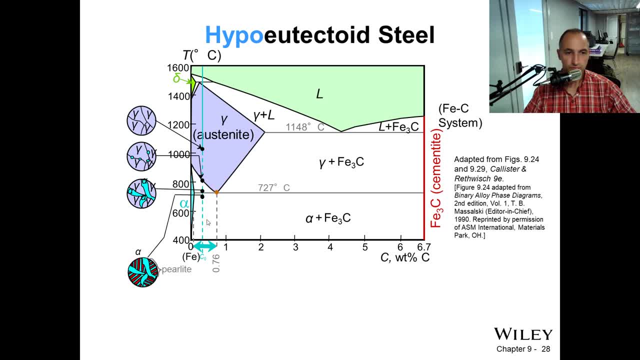 at which point you're going to get all solid or, I'm sorry, you're going to get all of that austenite transforming into pearlite. all the remaining austenite forms pearlite and a microstructure that is shown here. You have the pro eutectoid. ferrite pro in this case means the phase before the eutectoid. 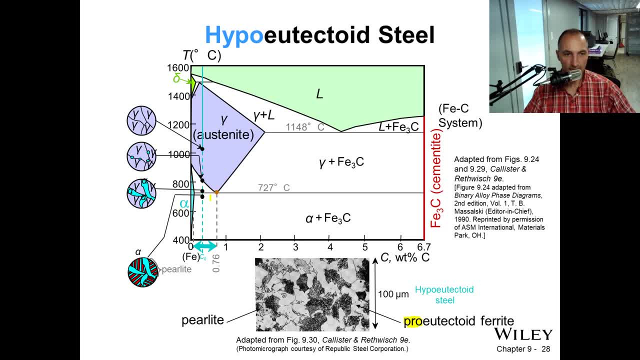 temperature. So that's all the primary or pro pro eutectoid ferrite. That's that light phase in here and it's surrounded by the pearlite, which is this darker gray phase here. that is what used to be the austenite. 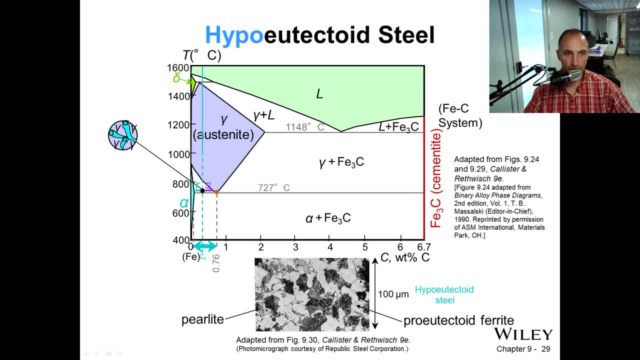 all right. so let's look at the weight, or first the composition of the. we're looking at the weight, the weight percent of alpha, and the weight percent of the austenite, the weight percent of the alpha at point. at that point there is just as over R plus S. 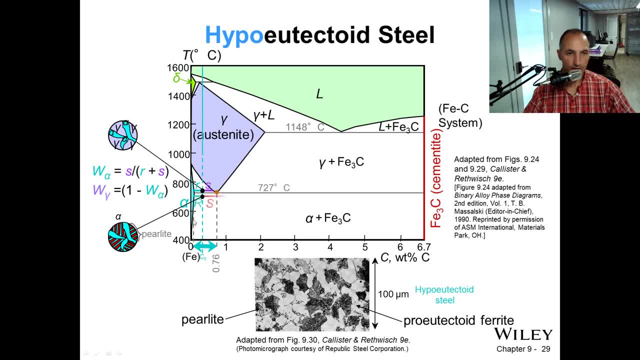 and then if, if we look at the weight percent of the Perlite, which is also the weight percent of the austenite, that is S over our plus That's. so what I can do here is put alpha over r plus tart of Ag to equal our weight. so I do now have this. I know how to seemed to shift for these sides of the testing. it would be interesting to see if we could nice little dot in l to get see if we can allowed to move those things a lot like Erva again. so we, you know. so it's all there, I get those things in place and the name is just a this part. so so 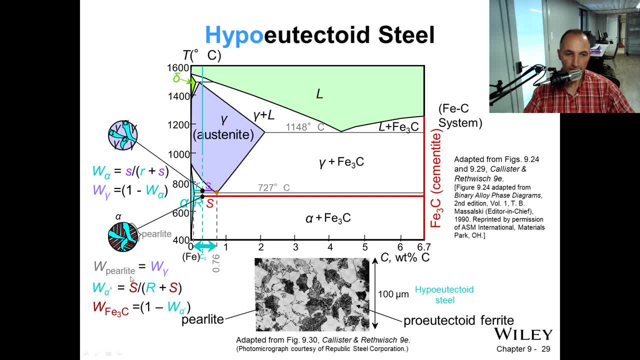 the weight percent of alpha is S over R plus S, so then the weight percent of the iron carbide is just one minus that, because, remember, everything in this area here, everything in this area here, is alpha plus iron carbide. so this is the weight percent of the iron carbide, and so that includes the 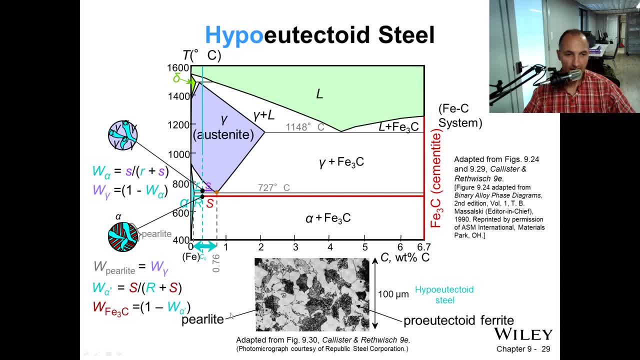 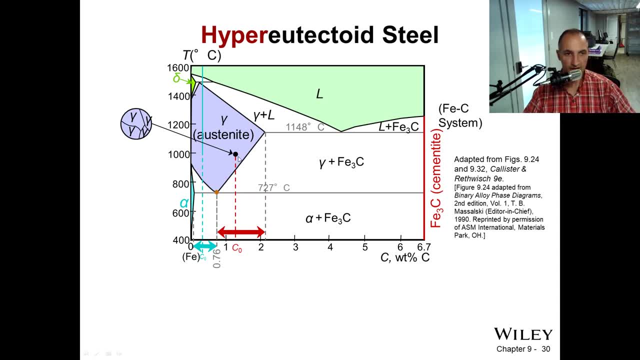 iron carbide in the pearlite and the weight percent. okay, so let's just move on to the next one. here I think I covered that good- the hyper eutectic, hyper meaning above eutectoid point. we start out with all austenite. 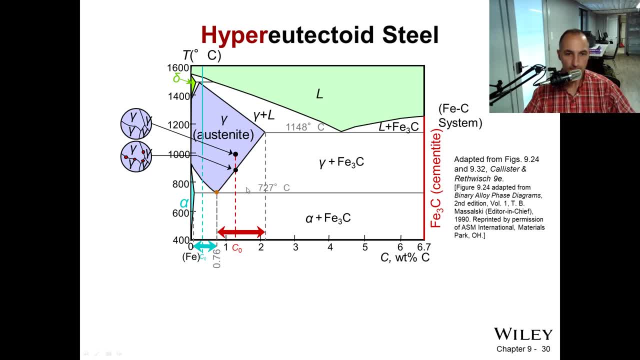 we're forming precipitates of iron carbide and as we continue to cool, the iron carbide grows and grows and then all the remaining austenite converts to pearlite. so the iron carbide, the weight percent of the iron carbide, is just um the X, X over V plus X. 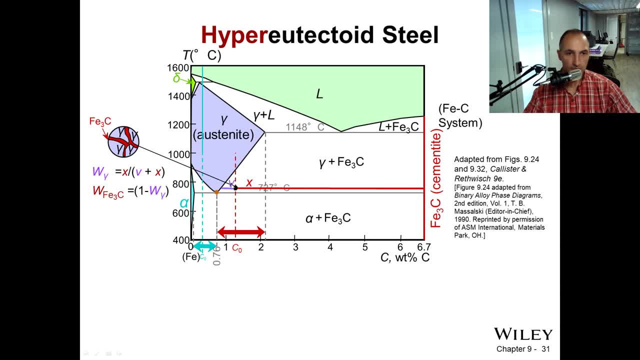 that's the weight-percent of the Alpha. remember, it's the opposite line, the weight percent alpha: X over V plus X and then one minus. that is the weight percent of iron carbide. so the weight percent of the, the austenite, ends up becoming the weight percent of the perlite. same. 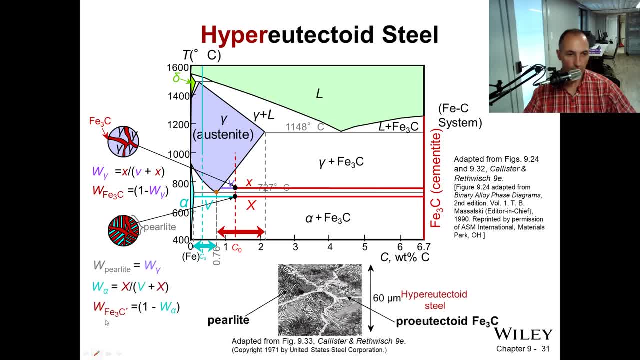 so weight percent. that's why I wrote it here: the weight percent of the austenite equals the weight percent of the perlite and then. so all we're left with having to determine now is what is the weight percent of the alpha, which is X big, X over, big X plus V, and then 1 minus. that is the weight percent of the. 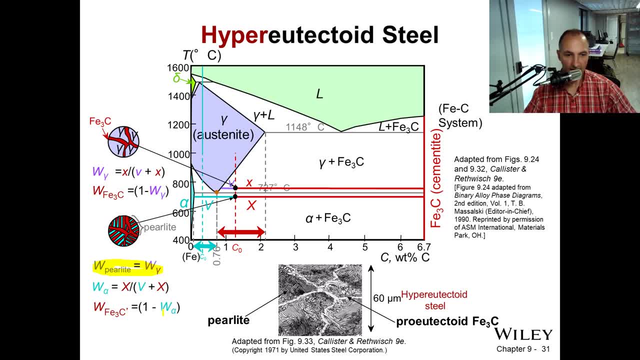 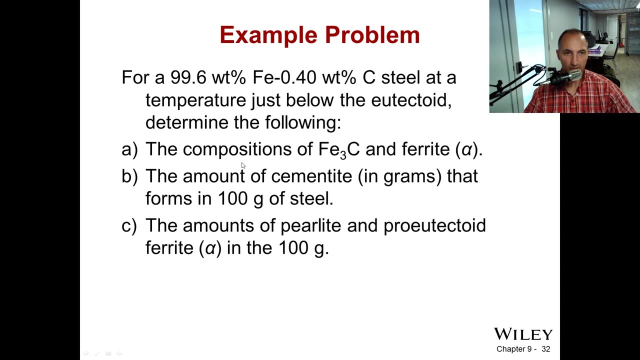 iron carbide and the weight percent of the iron carbide includes the iron carbide in the pro eutectic iron carbide plus the iron carbide that's in the perlite. so let's look at an example problem. we have 99.6 weight percent of the perlite and then the weight percent of the. 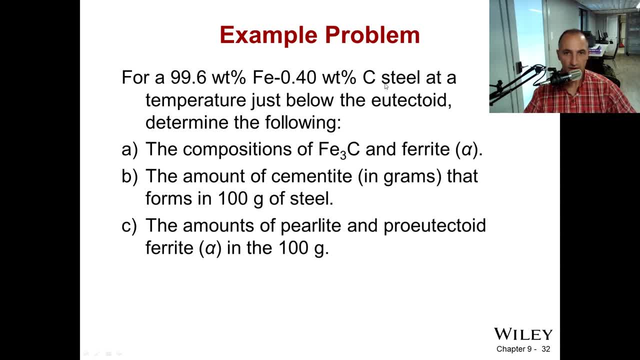 iron is 0.4 weight percent of carbon in a temperature just below the eutectoid. so determine the following: the composition of the iron carbide and the ferrite, the amount of cementite in grams that forms in 100 grams of steel and the amount of. 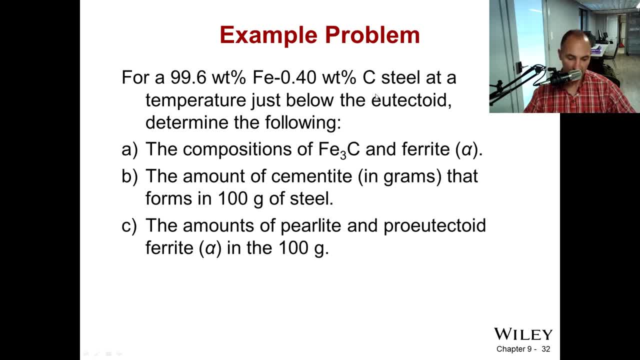 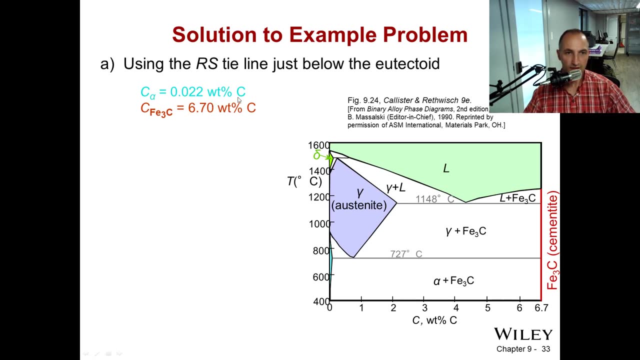 perlite and pro eutectoid ferrite alpha in 100 grams of steel. let's start with a. remember: a is the composition of the iron carbide in the ferrite. so the composition of the alpha using the RS tie line is 0.022 weight percent of carbon and 6.7 weight percent of iron carbide. 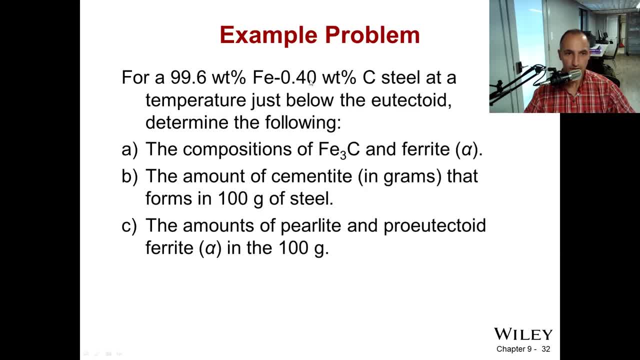 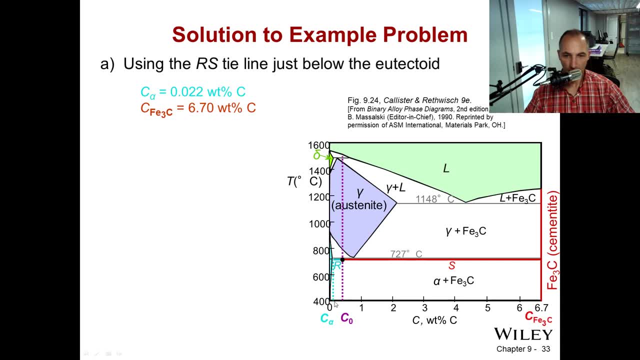 going back to here, remember we're looking at a 0.4 weight percent, so that's this is 0.4. right here, remember, this is like a really small composite. this is only 1, 1% copper, so this would be like 0.5. so this is 0.4. 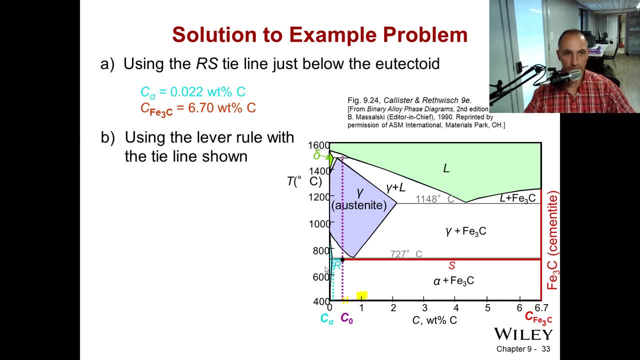 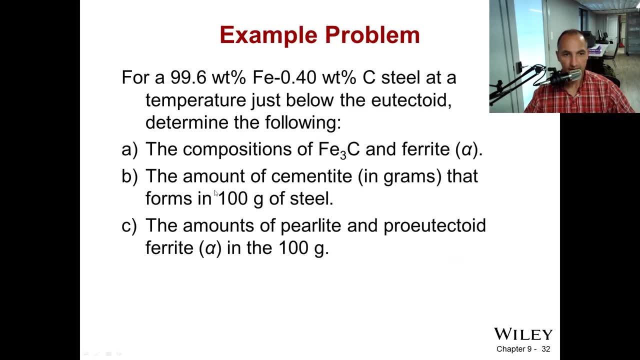 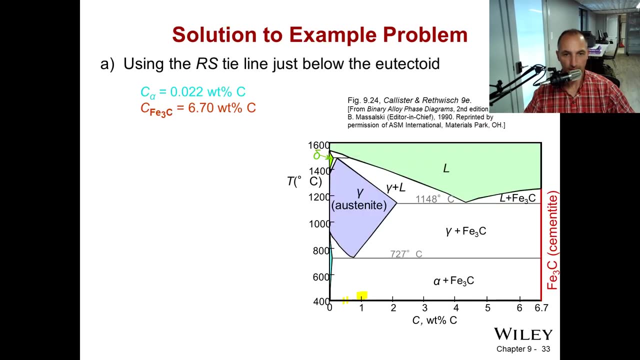 so that's why we drew that line right there. using the lever rule, we can determine B and we can determine B and we can determine B. remember, B is the amount of cementite that forms in 100 grams of steel. so first thing we need to do is find the weight, percent of cementite, the weight. 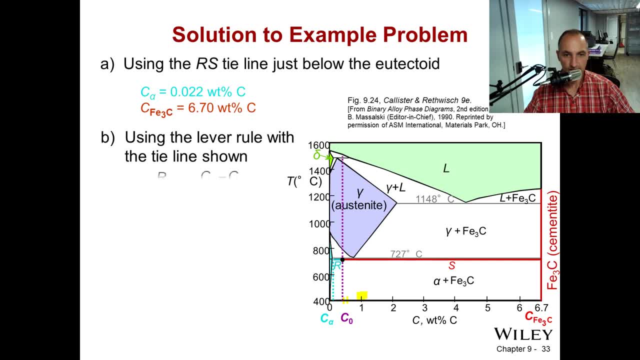 percent of cementite is just the lever rule got to do that, and so the lever rule is just R over R plus S. the opposite of where cementite is. cementite is all the way over here to the right, so we need to find the length of the line. 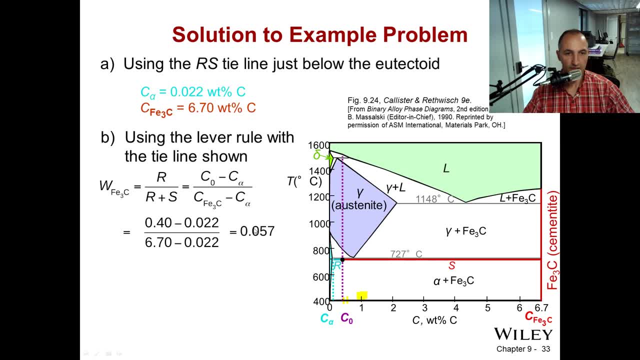 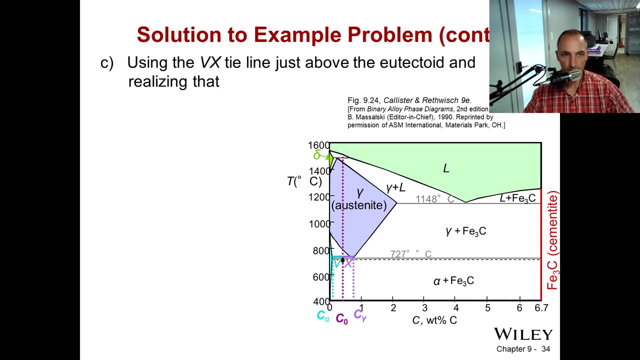 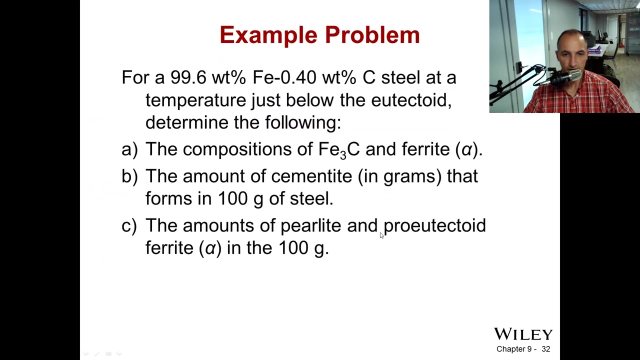 on the other side and that is point zero, five, seven percent. so take that number and multiply it by a hundred. this is a hundred grams and that's going to give us five point seven grams of iron carbide in the 100 grams total. so question C: going back, question C was the amount, the amounts of perlite, sorry. 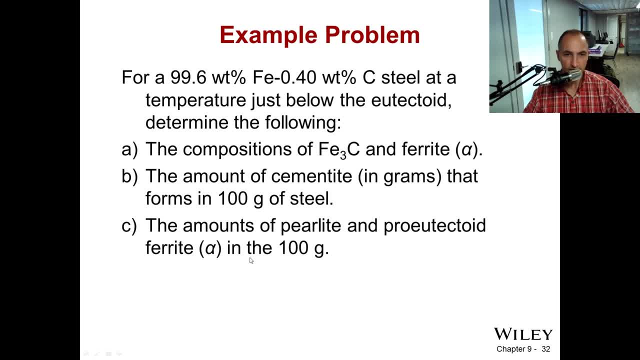 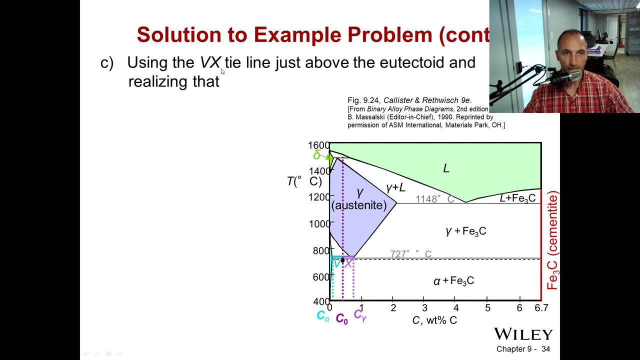 the amounts of perlite and pro-eutectoid alpha in 100 grams. so again, this is a weight percent information that we need to get. so we've got to use the tie line BX tie line just above the eutectoid and realize that the composition, overall composition, is being point four. we know. 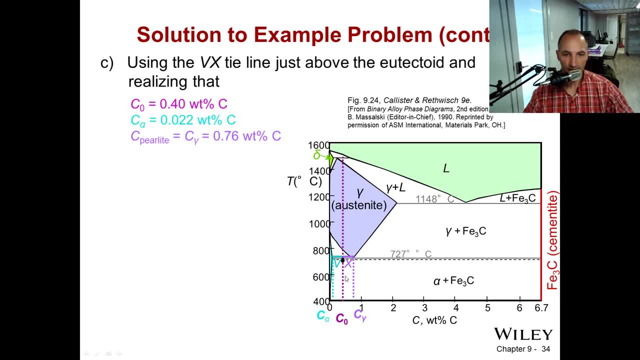 that the composition of alpha is point zero, two, two get that. and the composition of the perlite is also the composition of the austenite, and that's 0.76 W percent. so the composition just above is also equal to the composition just below. so that's where. 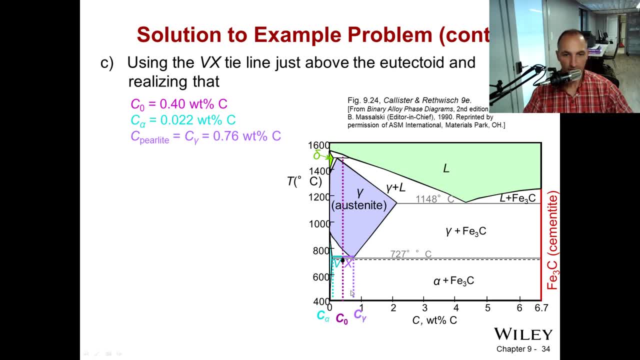 we get this C gamma here of 0.76. so now we got to get the weight percent of the pearlite. weight percent of the pearlite exactly the same as what the weight percent of the austenite was, just above the eutectic temperature. so that's just. 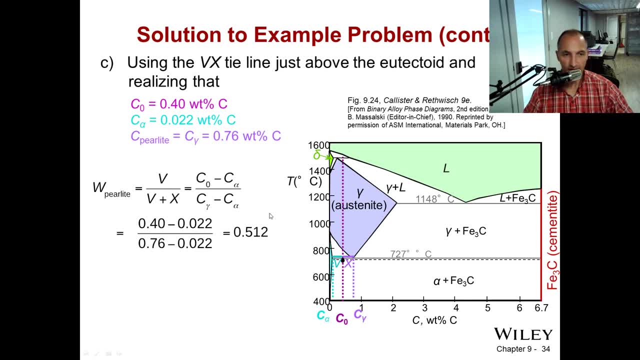 Vx, I'm sorry, V over V plus X, so that's C C0 minus C alpha over C gamma minus C alpha, or 0.512 weight percent. again, take that percentage, or we take that fraction, multiply it by 100, and now we have 51.2. 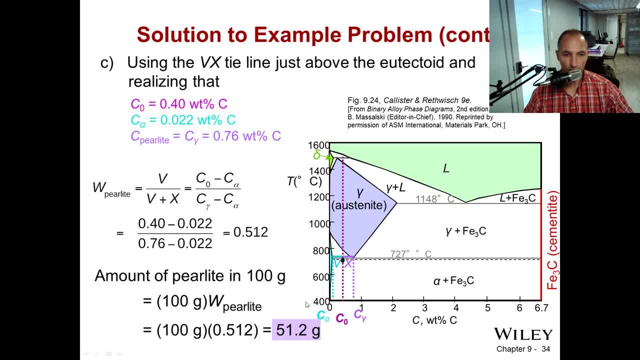